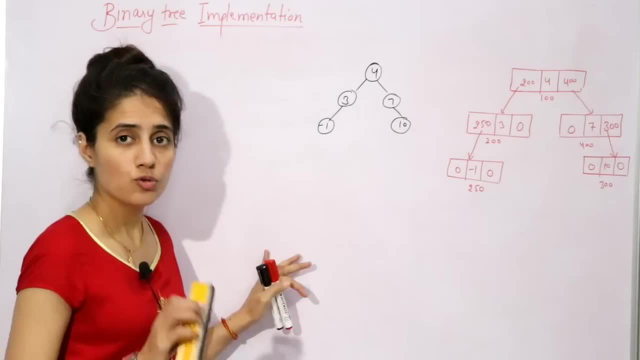 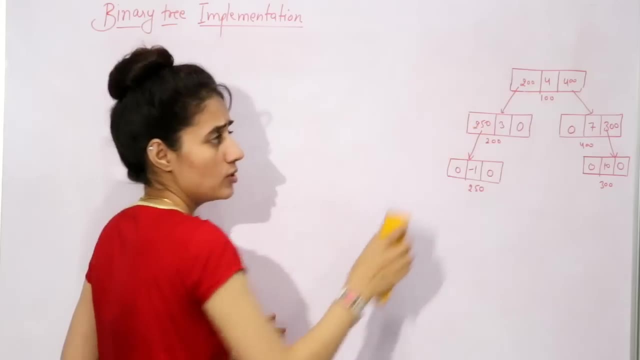 Meaning: this is the left child, This is the left child, This is the left child, This is the left. So what you are going toTO create this binary tree right See. now see what nodes, how we are going to create the nodes that we have already discussed when we were discussing the linked list. 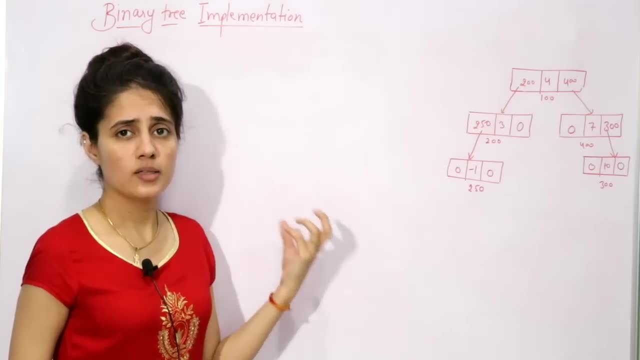 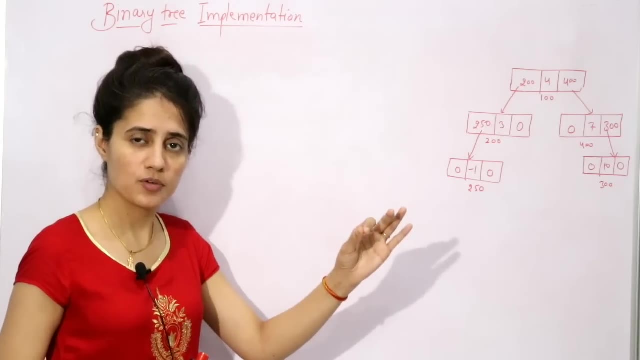 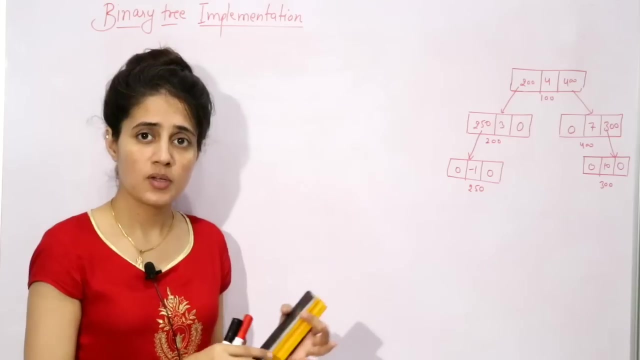 implementation right. So now this is what they're going to: dynamically allocate the memory to these nodes. Fine, In the list, in the linked list, we always maintain what the head pointed by the head pointer. you can easily traverse all the nodes of the linked list same in the same way in. 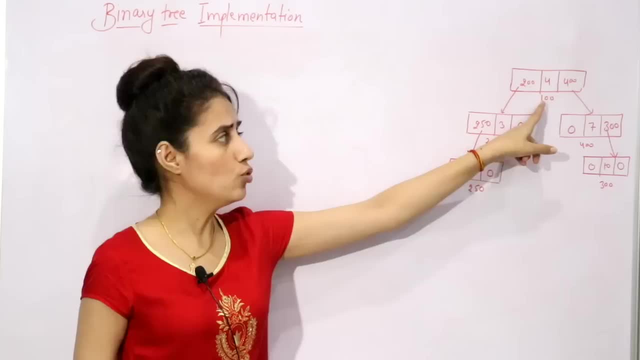 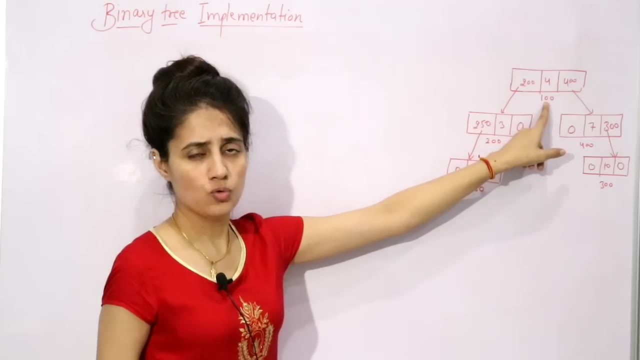 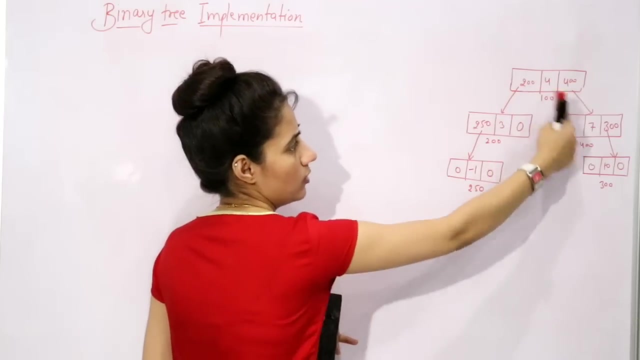 the tree. we have what we will have with us: the root pointer or you can say the pointer to the root node. right here we will contain what this one address of this root node, that is 100. if you have the address of the root node then you can easily traverse all the nodes from the root node right. 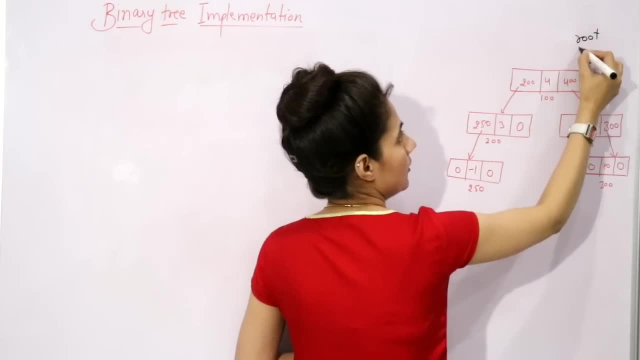 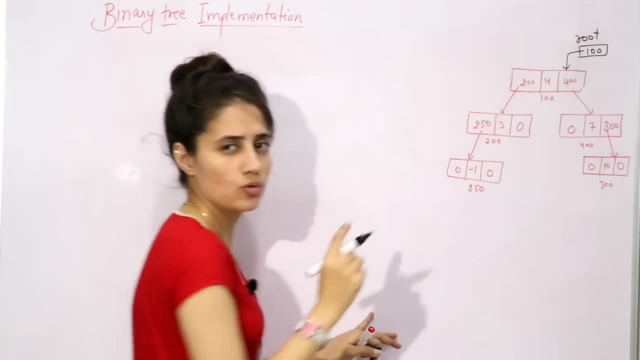 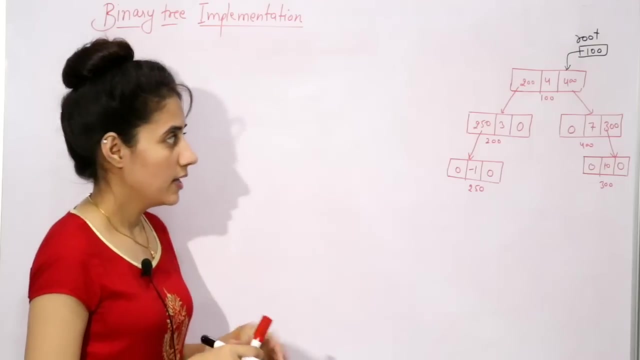 so here we have what you can say, a pointer, root pointer, and there we are going to store this one hundred address of this one right, and we just maintain this root. here i am taking the name only root, but this is what a pointer, not root node, this is what the root node. so now see here: 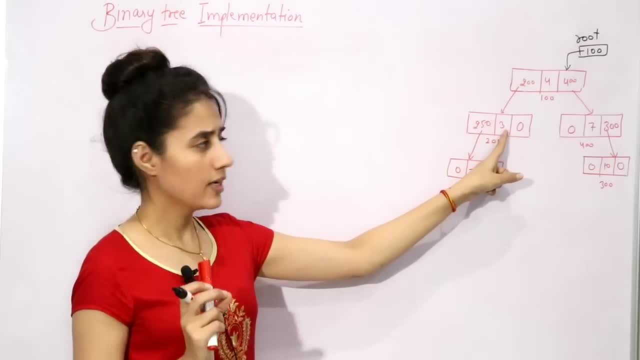 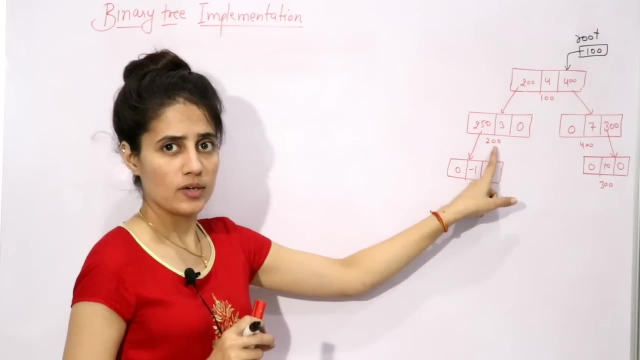 each node is having what? the data part that is integer, the data type of this is integer and data type of this, and this is what these are pointers, right? so these are pointers to node. fine, so now you have, we are going to define your own data type. that already we have discussed in linked list implementation. so this: 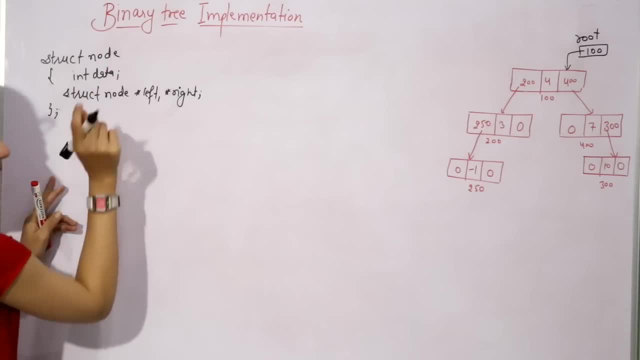 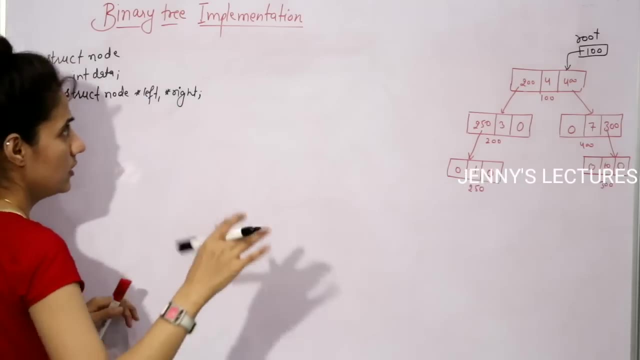 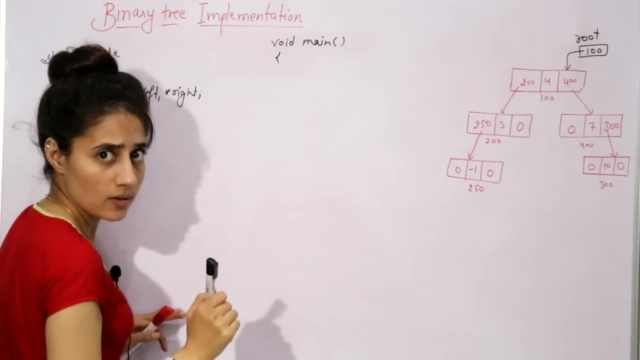 is how we are going to define our own data type three parts. struct node is the data type three parts is there. one is data part and two are left pointer and one is right pointer. right now see in main function what you will call. we are going to create this tree, right. 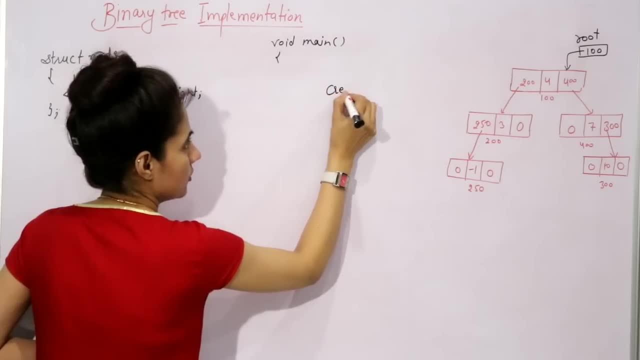 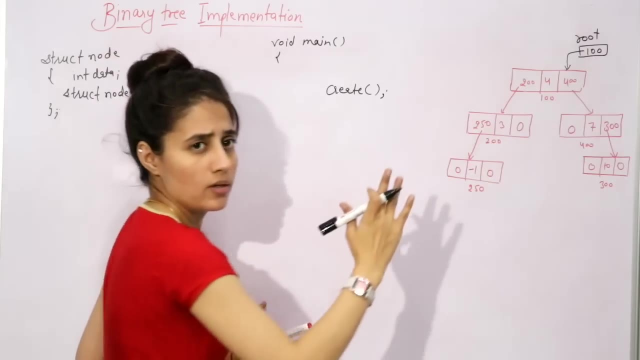 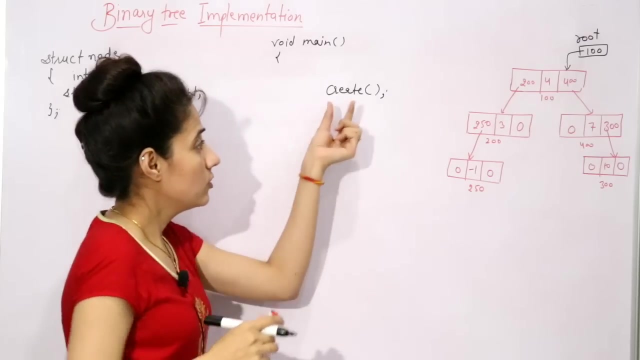 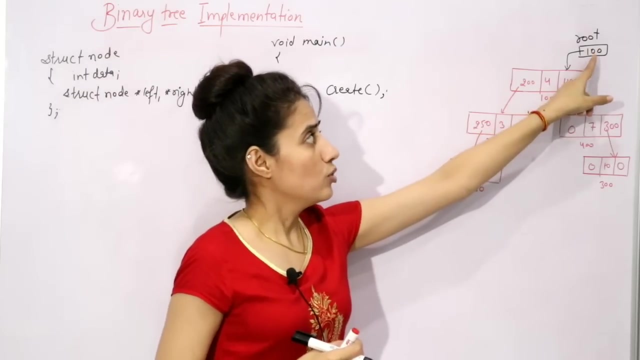 so now in main function we are going to call what create function, fine. now what we want after creating this tree, what you are going to store, this value, that this address, that is hundred, fine. so now i want this, this root, the sorry, this create function would return this hundred, this pointer right. so the pointer is what this pointer is? pointer to node. 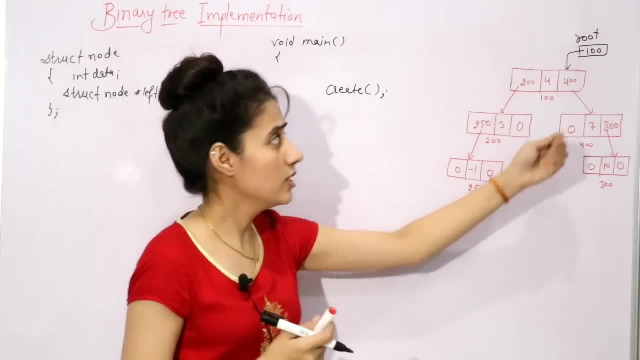 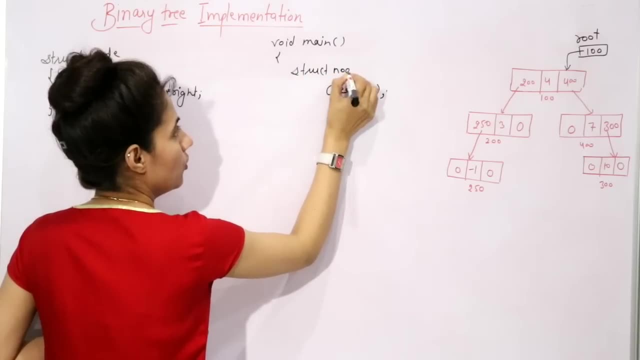 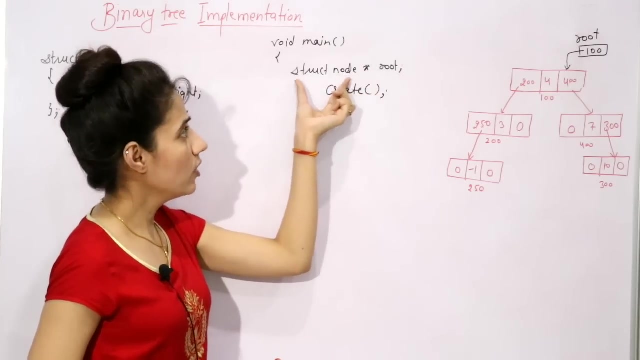 pointer to this node, struct node. so obviously you are going to define this pointer first of all. right, so here, first of all, you will write struct node, asterisk root. so now, here asterisk means this is the pointer, and here why you are writing this: struck node. 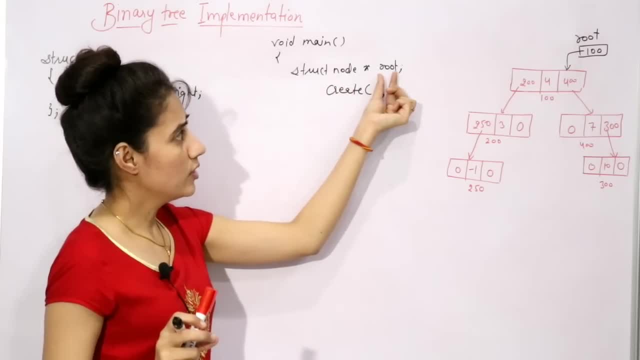 this thing also we have discussed many times. see, this root is containing address of this node and here, always, you will write what the data type of that variable whose address this pointer is going to store. this pointer is going to store address of this node and data type of. 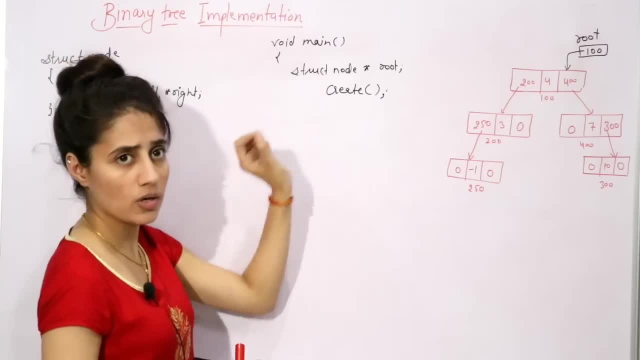 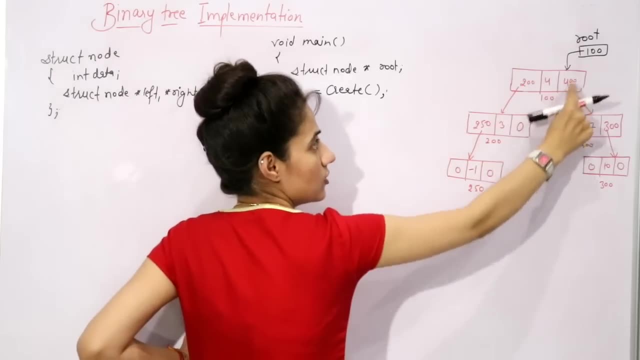 this node is. we have already defined this node, exposing strata of this node. so 10 of this node, that is struct node. that is why here i am writing struct node. now, whatever this, create will return means create will return. what address of this node that i am going to store in root? so here: 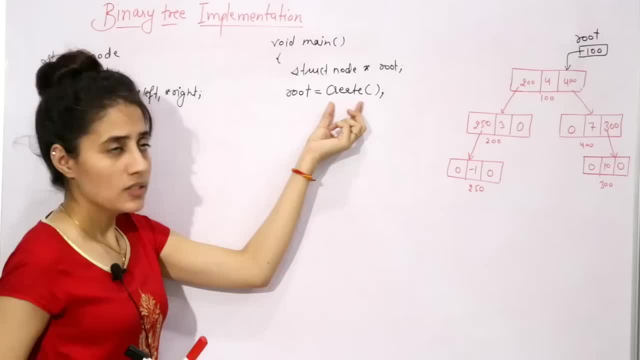 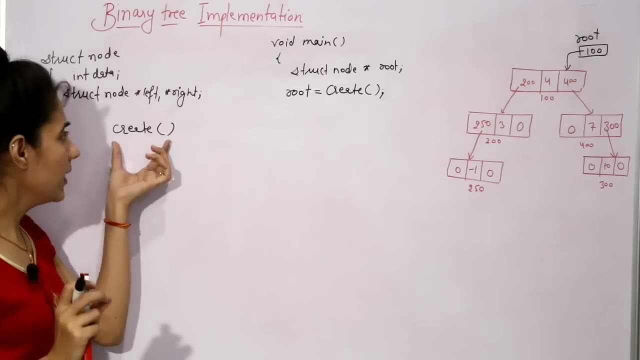 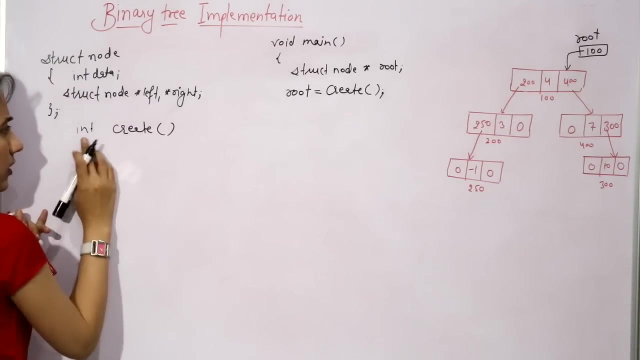 you will write what root. so now this is what calling of this create function. now we are going to define this create function right. see now what should be the data type of this create function. see when a function will return integer type, then always we type here, we write here: int if function. 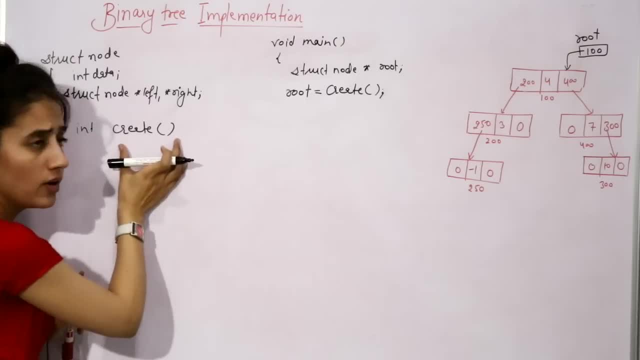 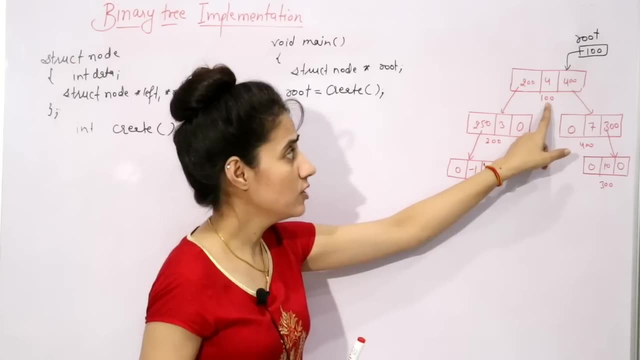 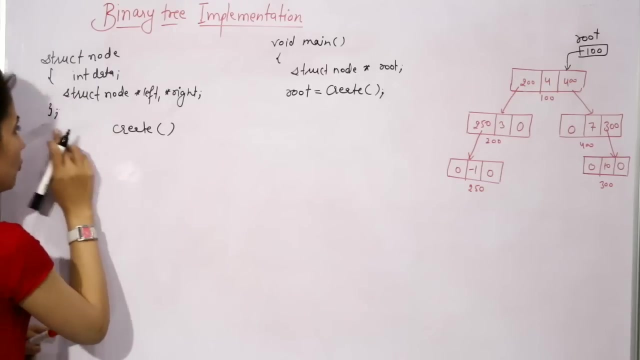 does not return anything, then we write here: void. but now this function is going to return what address of this node, right? so this is going to return what pointer value, but you can say: pointer to this node, pointer to this node. so now what data type you should write here? 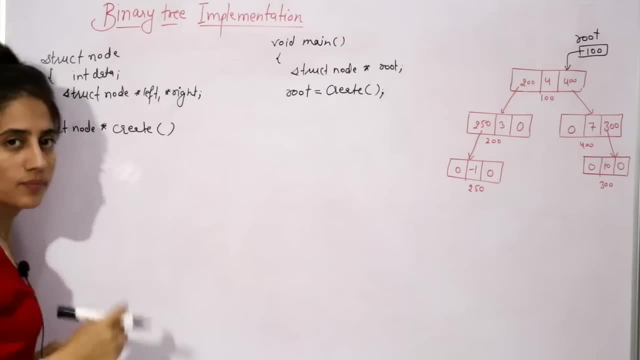 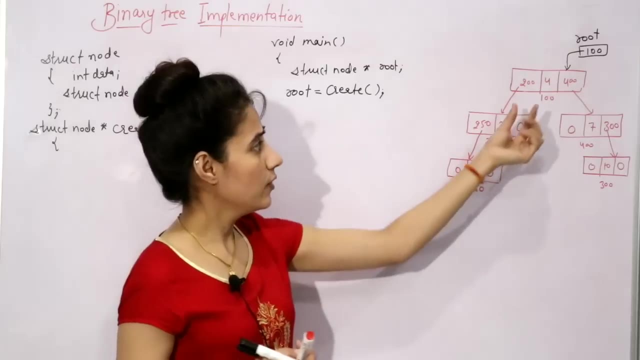 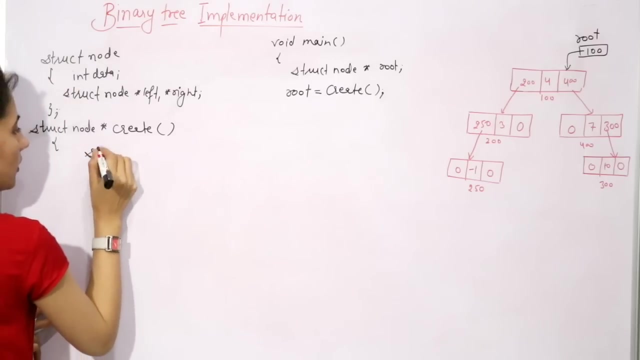 struct node a streak, because it is going to return pointer to node. so now for inserting these values in the tree. first of all, we are going to create this node right and you are supposed to dynamically allocate the memory to these nodes. so now here see this thing already we have discussed. 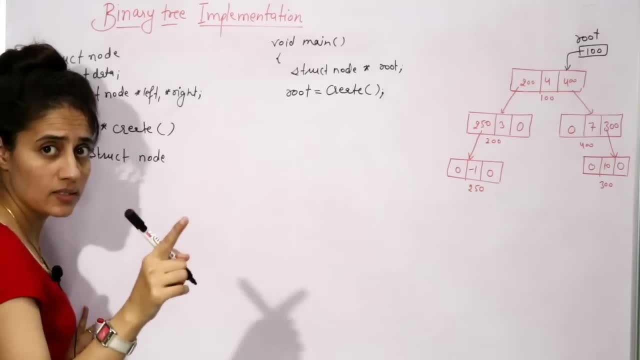 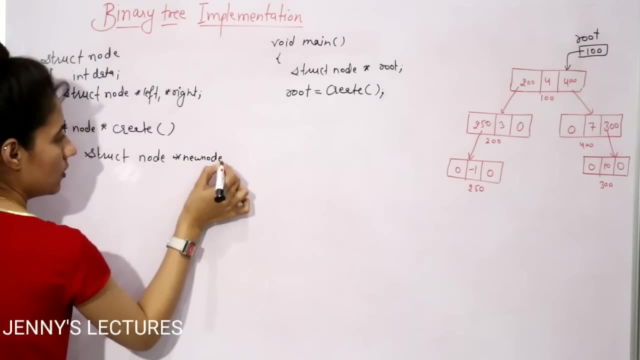 when we were discussing the implementation- sorry, the linked list in the data structure. many times you have discussed this thing. so first of all, you are going to create a node. you can say you can take a new node and dynamically how you are going to allocate the memory using malloc function in c in. 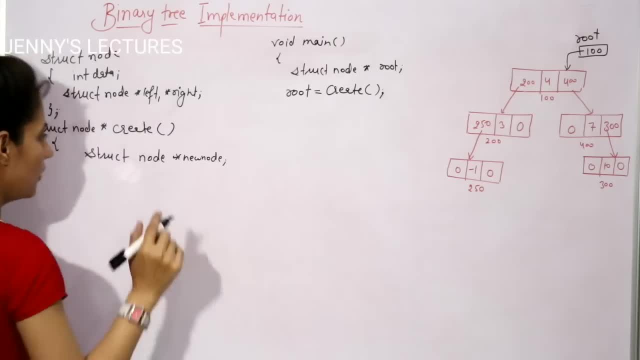 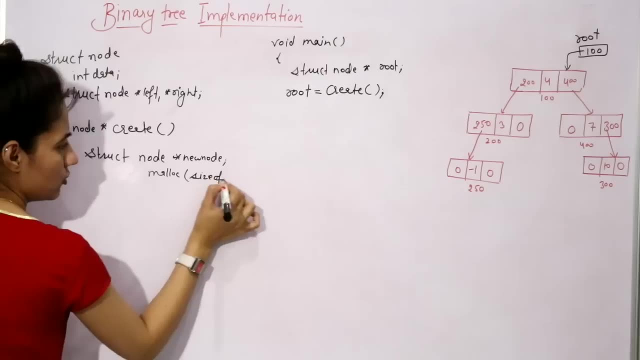 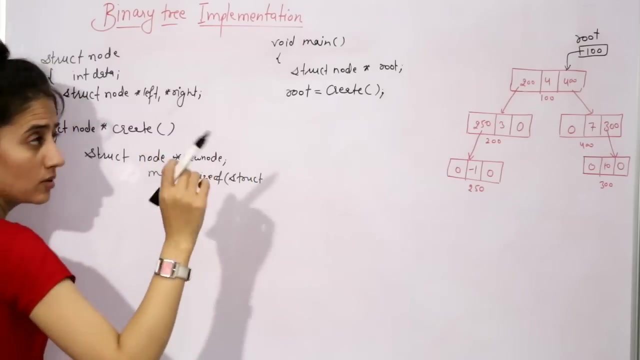 c plus plus. we will use what? that new keyword, fine, and the syntax also. we have discussed many times malloc. here you will write size of keyword and size of this one. for this node i want how many bytes see that. you will write here the data type of this node, that is struct node. the data type is struct node. 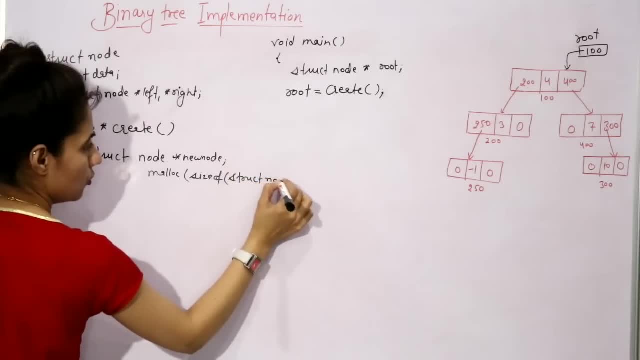 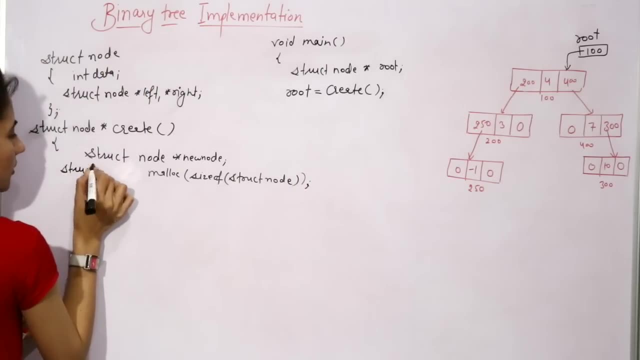 you will write here the data type of this node, that is struct node. the data type is struct node now, now this malloc is going to return the void pointer, but here this new node is what this is pointer to a node. so you have to typecast this thing and whatever this will return, we are going. 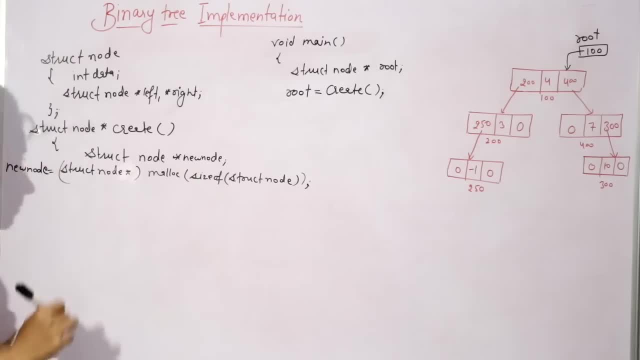 to store in new node and now we will ask for the value from the user, which value he wants to insert in that tree using printf and scanf. so you need some variable to store that value. suppose i am taking x, so here you need to declare this variable, int x right now. suppose here. see, here i don't want. 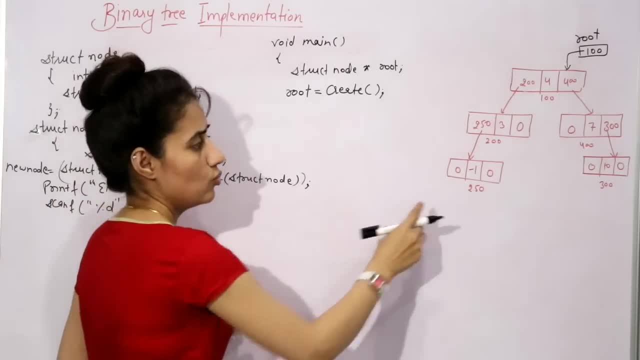 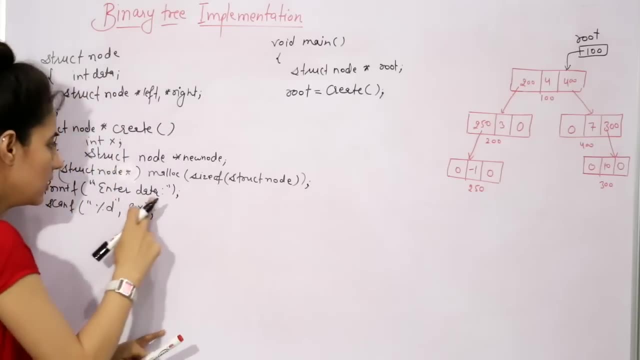 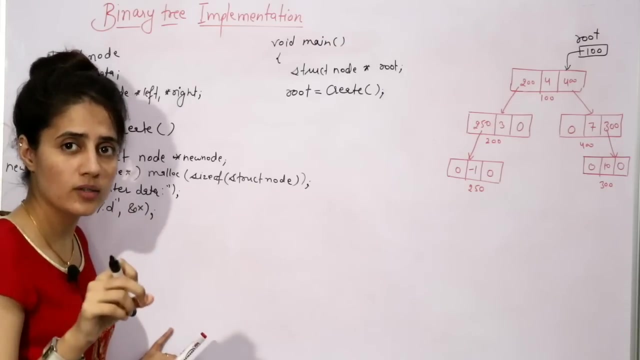 to insert any node further. fine, so how we are going to write down that condition, that base condition, returning condition. so suppose, when you are entering the data, if you don't want to enter any child, so you can insert simply minus one, and if you have entered minus one, then simply it will. 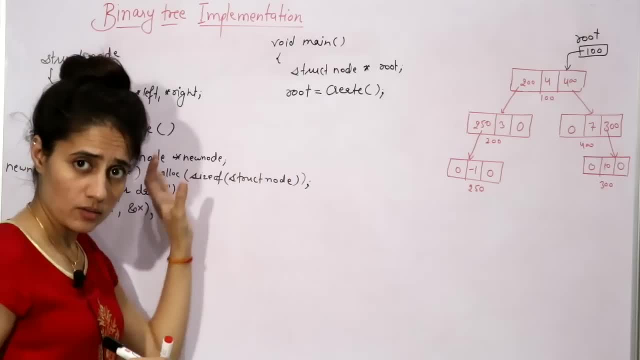 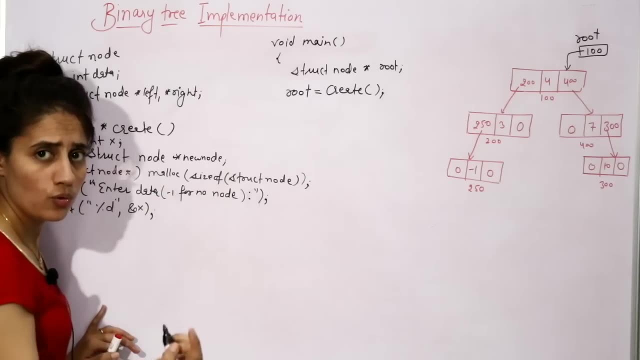 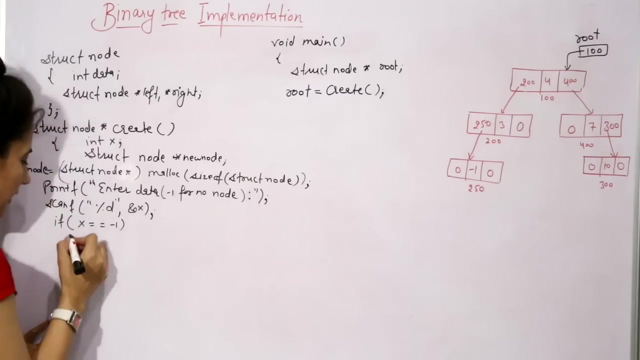 return zero, or you can say null, the. thus this execution also i'm going to show you fine. so here, simply you can write: enter minus one for no node, right. and here you can check one condition: if x is equal to, is equal to minus one, in that case, simply, you are going to return zero, or you can 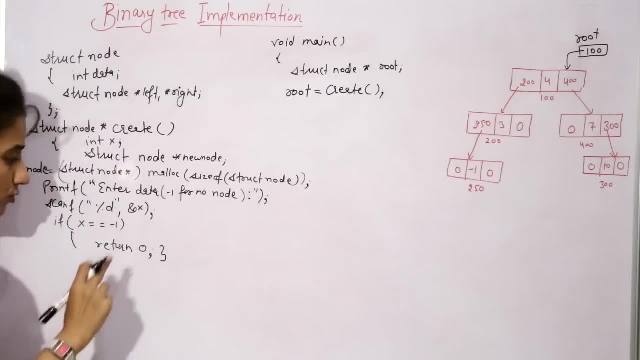 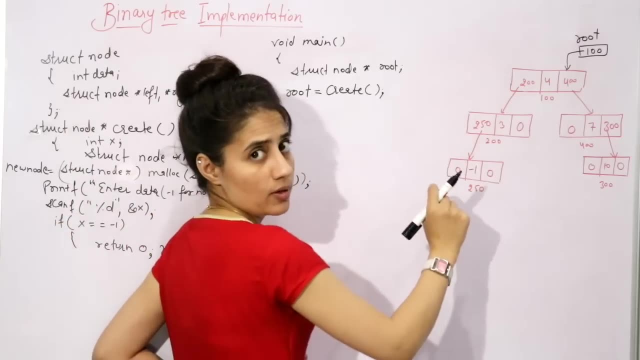 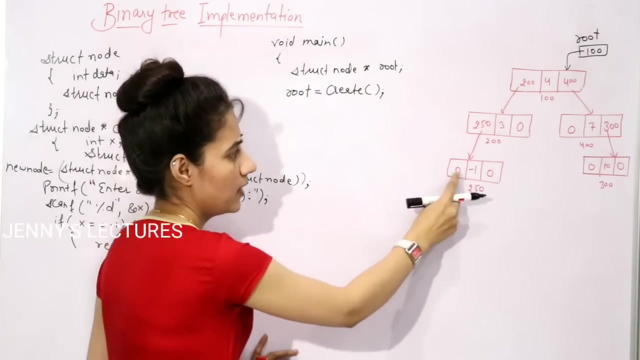 say null, right, else now you are going to write down what see. now see, here, in this case we are going to use what recursion? because suppose we have entered four, then the left child, you have entered three, then again the left child, again the left child, and once you don't want any left child, then here i don't want any left. 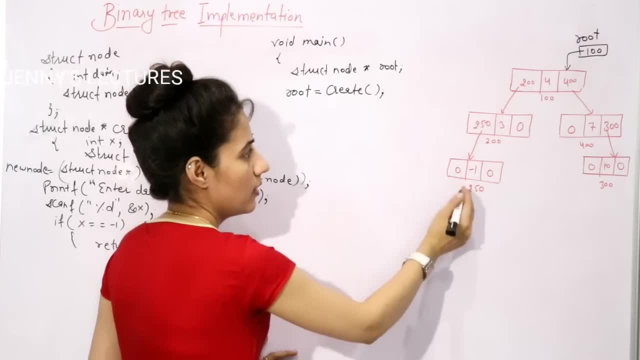 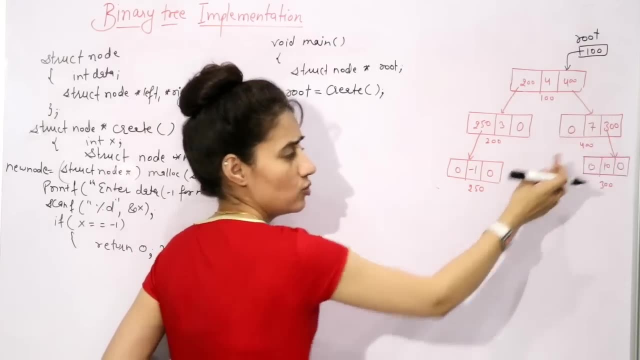 child. also, i don't want any right child. then back to here any right child you want. suppose you have entered minus. one means back to here here. i want that right child. so this is what a recursive call, this is what recursion. so the prerequisite for this video is what you need to know: what is a? 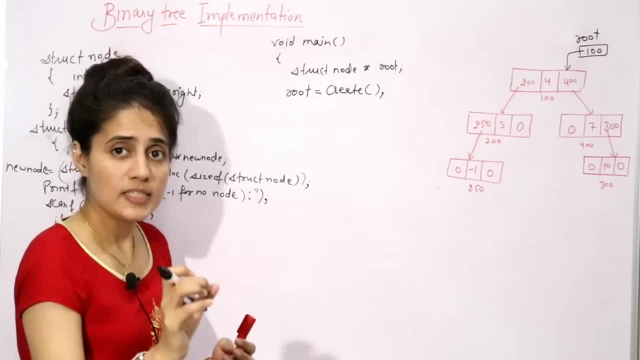 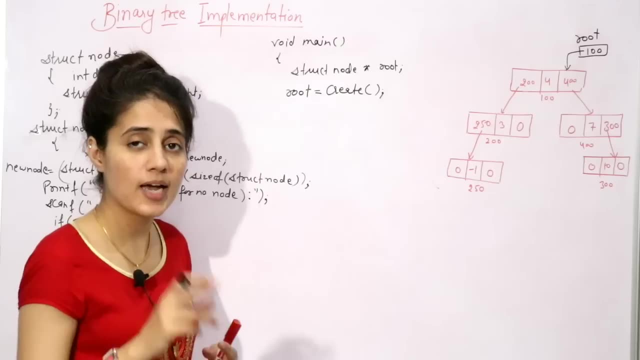 recursion and how recursion is a recursion and how recursion is a recursion and how recursion is a recursion is a recursion and how recursion works, works. or basically, you need to know how the avoid named memory is to be allocated when you are going to америк. exercises the recursion, that things are. 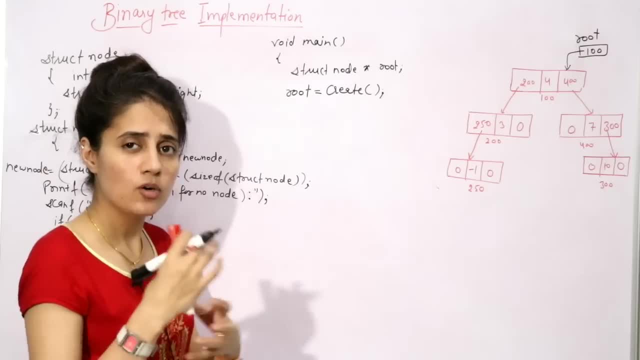 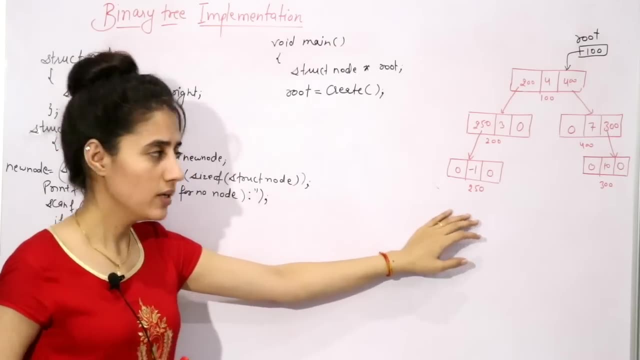 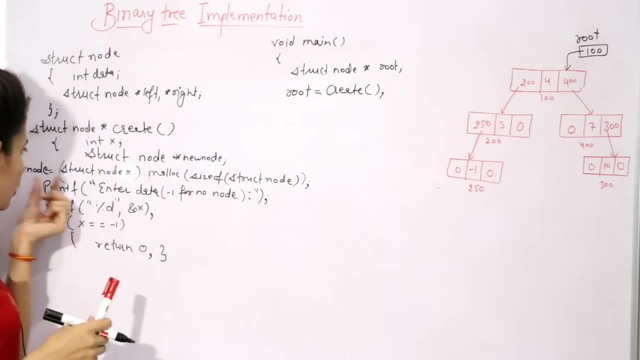 very important. if you know working of that recursion, the memory allocation in case of recursion, then you can easily understand the working of this binary tree implementation right. so now i have entered the data, supposed that data for now. if obviously you have created this new node, then initially this new node is what doesn't have anything close to this node. firstly, you have to add data to add this type of data to it. 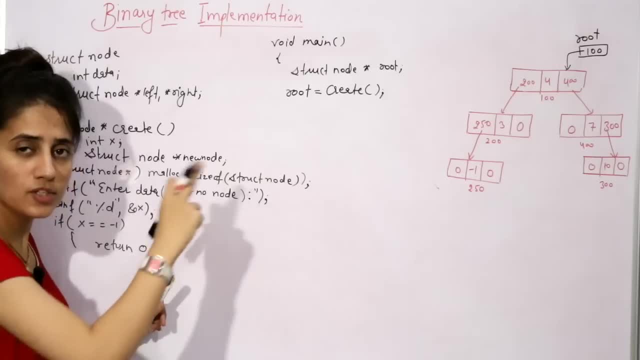 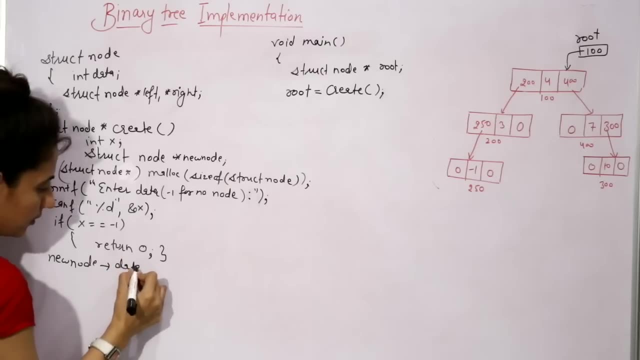 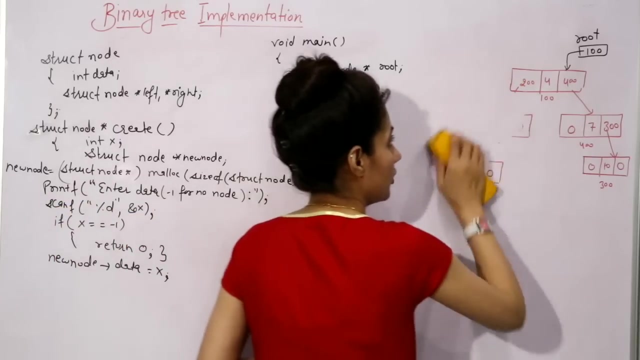 so you need, you need to store that value 4 in this new node, right? so here how you will write new node and in data part i will store x. fine, see, now i am going to rub this thing and i am going to tell you how this is going to work. see, this is how we have created this new node. 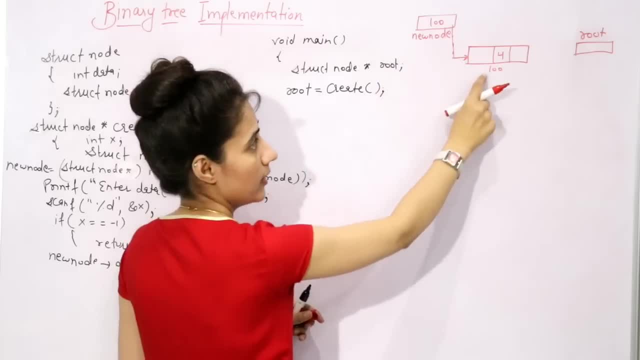 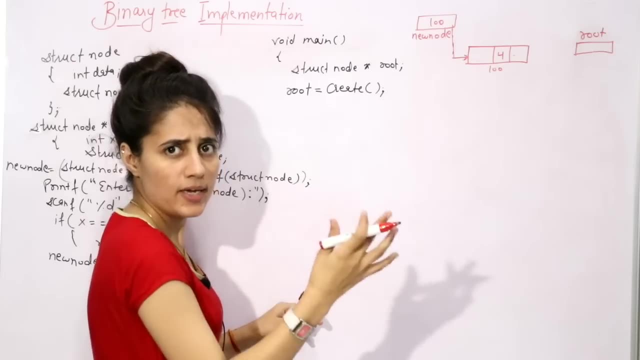 and address i have stored in this new node pointer, that is 100 suppose, and here i have stored in the data part 4. if you want, here you can store null and null and null, zero and zero. but here i am creating this tree because i want the left child also right child, also the, here i will store address. 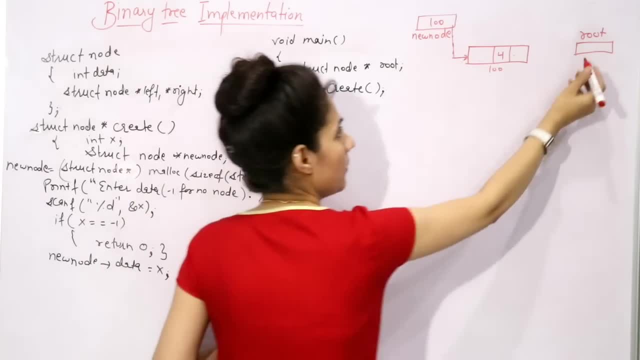 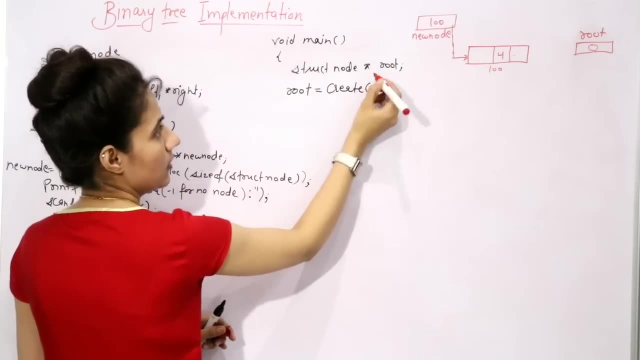 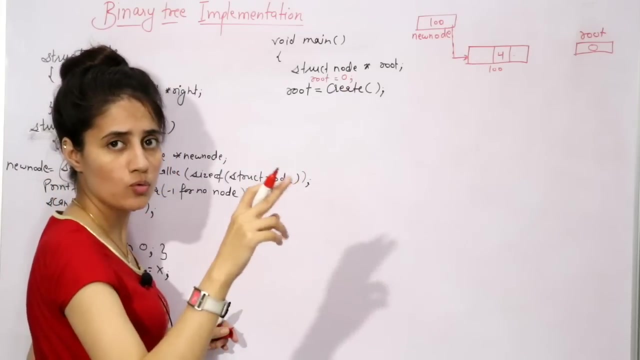 of the left child. that is why i am not storing here null initially. suppose i am storing in root also null right now, what you will do. so here you can write simply after creating this root pointer: here you can simply store: root is equal to zero or null. 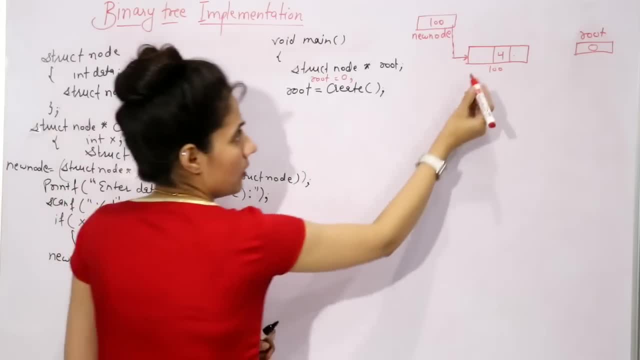 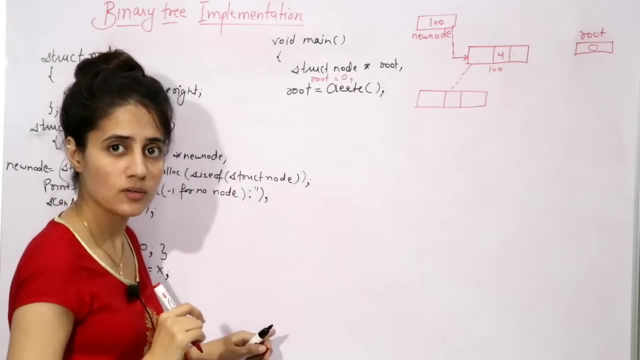 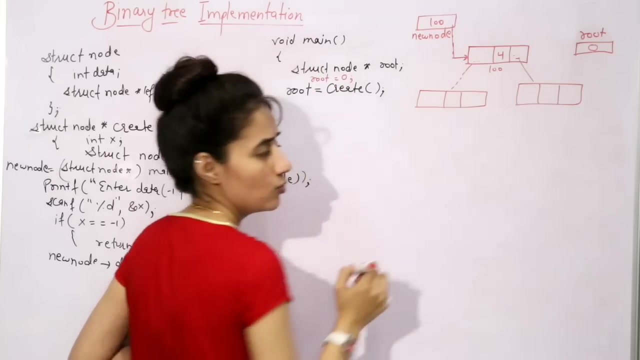 right now. see here: now i want to create a left child, so again you need to call create function. right, and also i want to create right child, so in right, here also you are going to call the create function. so within this create, i am again going to call create function. this is known. 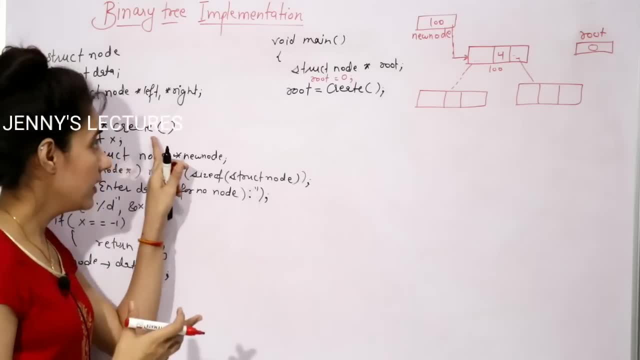 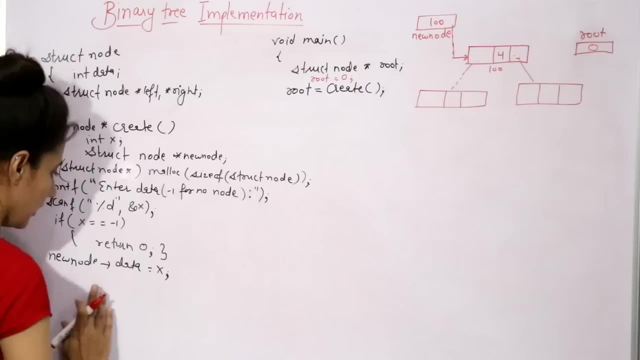 this is known as what recursion, because a function create is going to call itself itself again, right, so this is called a recursion. fine, now here, after storing the x value here, here i will ask from the user: enter the left child right. so here, simply, you will write: 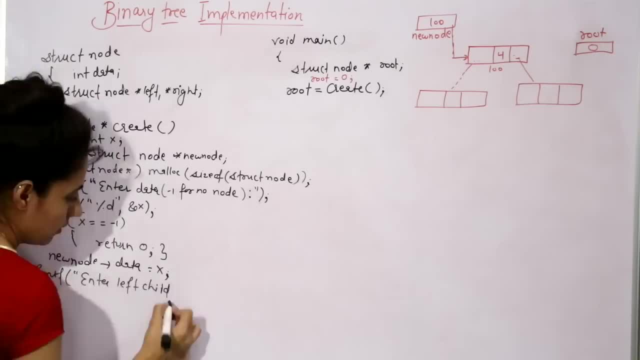 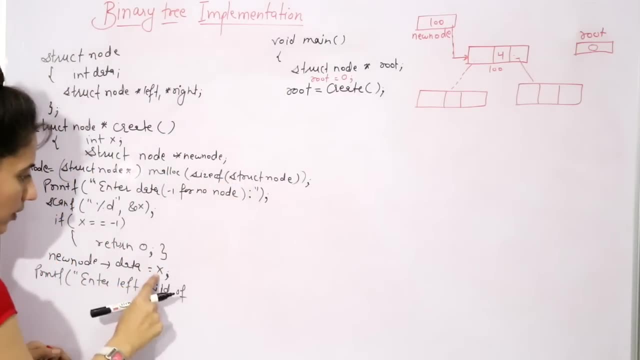 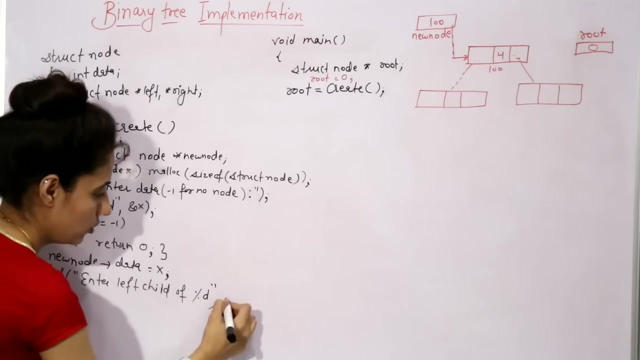 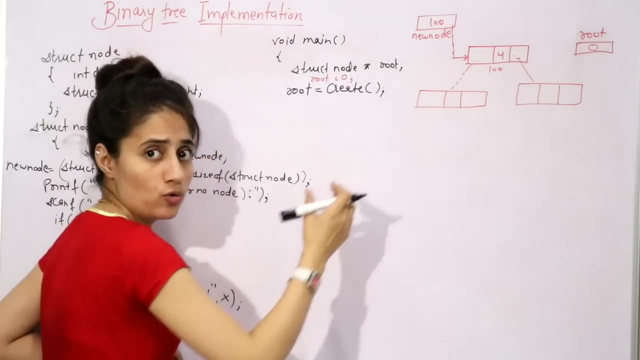 left child of this one, that is, left child of four, i want. and here now x value is four. so you can: here right, left child of sorry, here you will write percentage d and here you will write x means left child of four, right and here same. you are going to what? 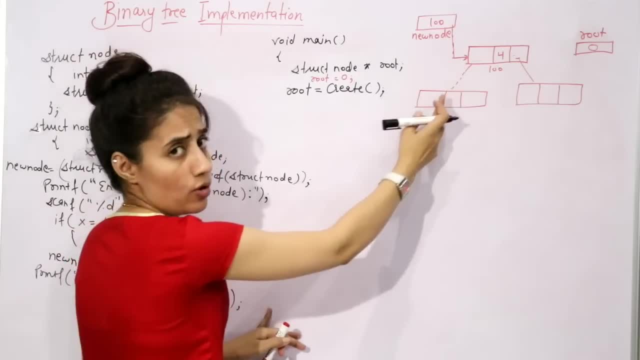 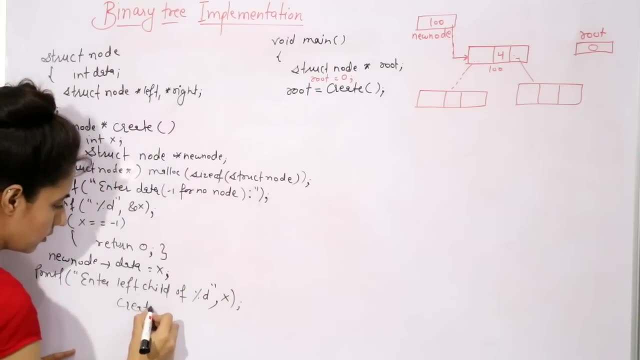 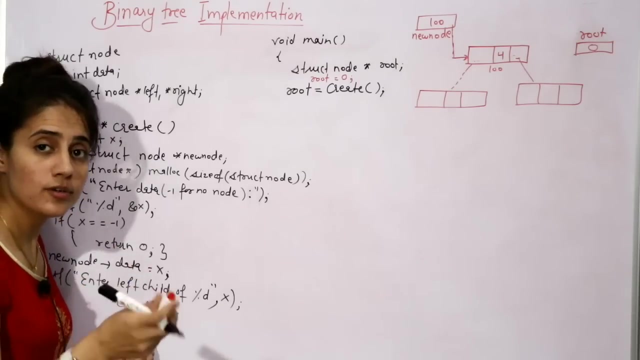 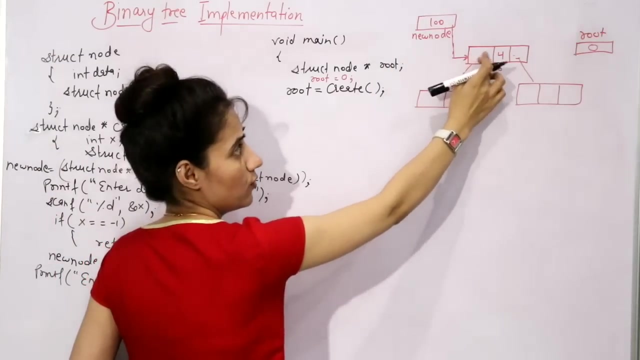 call this, this function, create function, because same processor i want here this node should be created right. so here simply you will call this create function again and what this create function is going to return. a pointer to node means: if you call create function here, here i am calling to the left of this one, left child of this one, here i am. 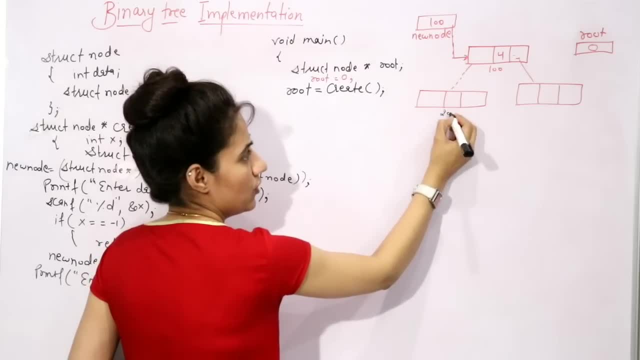 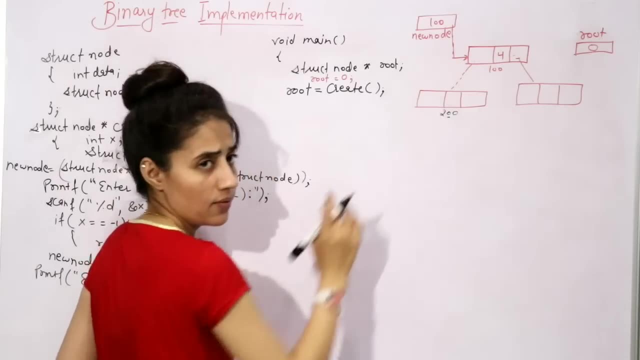 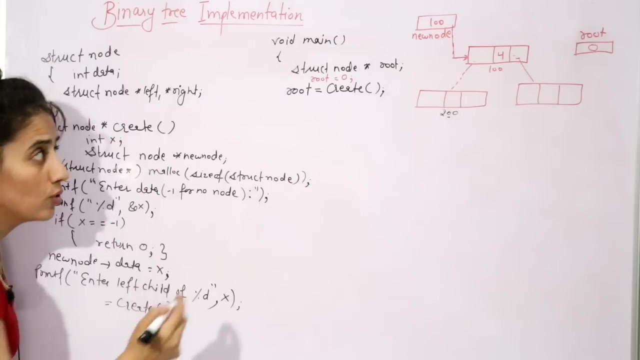 calling that create function. so suppose the address of this one is 200, so it should return 200 so that i can store this 200 here. obviously i want to store this address here, right? so now see, whatever this create function will return where you are going to store here. that is new node left. 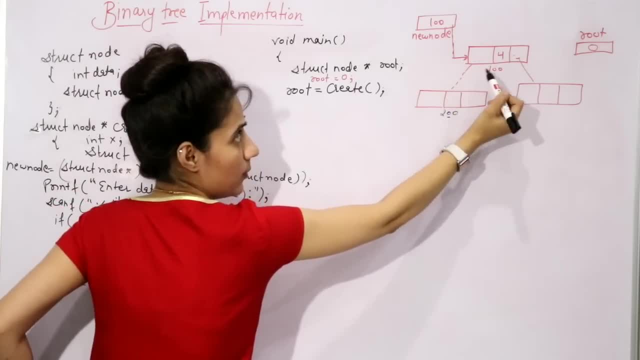 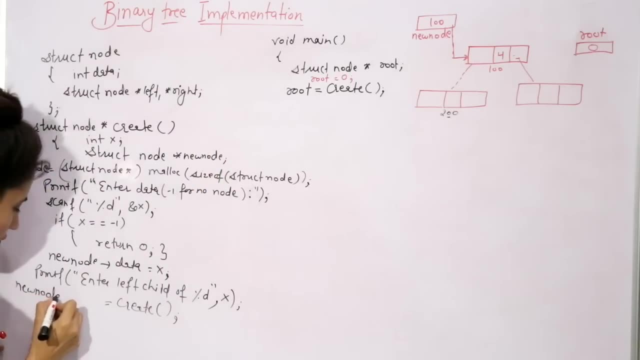 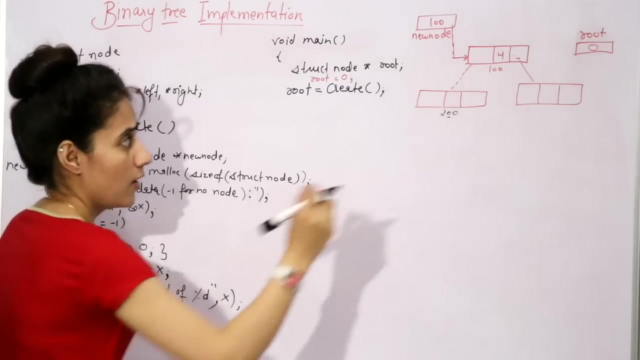 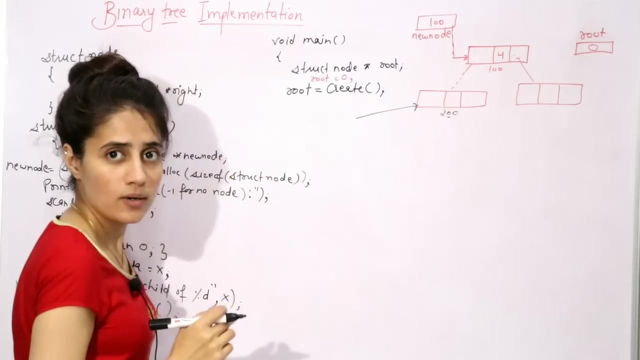 right, because to access this node you need a pointer, and pointer to this node is new node right. so here, simply, you will write new node left right now. see, please do not get confused: after creating this node, that new node is going to point here, so this new node is not going to point here. that is why I am saying you: 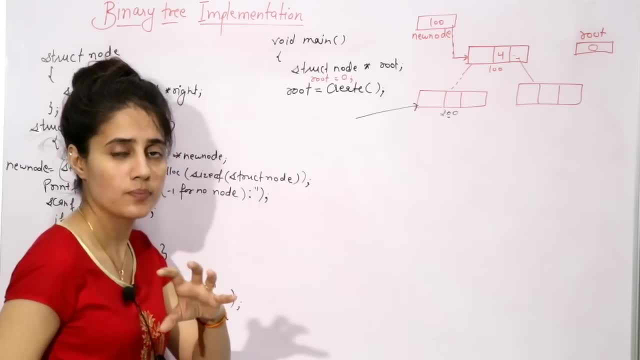 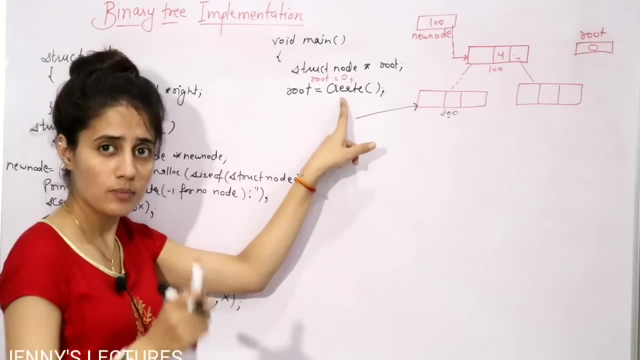 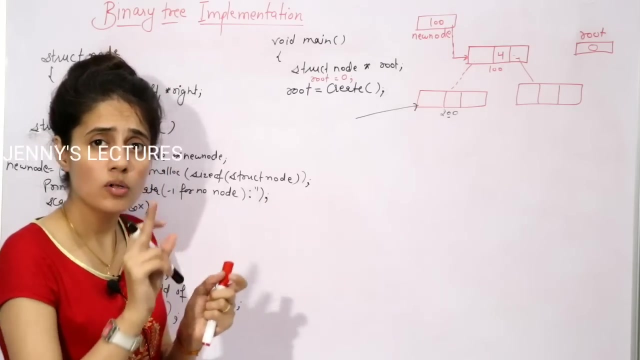 first of all, please read how the memory is to be allocated in the function call, because see when a function is called from the main function, then the memory is to be allocated to this function in the stack and the most important point is different copies of all the local variables would be created. 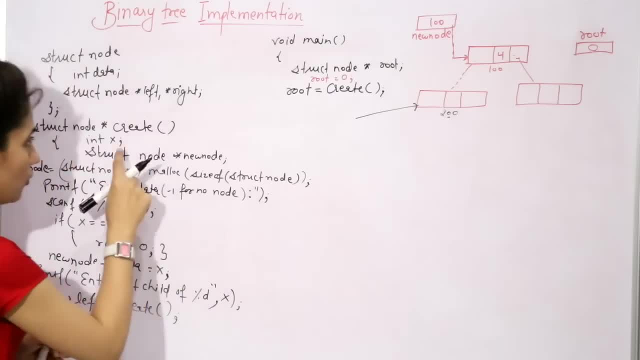 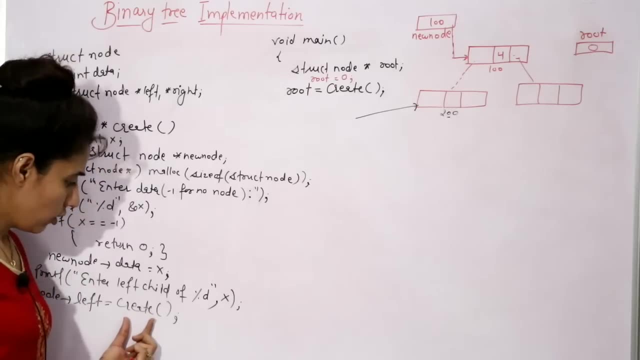 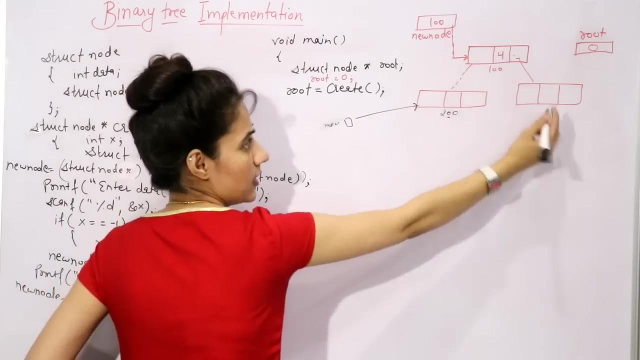 for each function call, right. so this is what X, this new node, these are what local variables, right? so whenever you are going to again call this create function, then one copy of this new node would be created here also. if you call at this side, then here also one copy of this new node, pointer, would be created. so here. 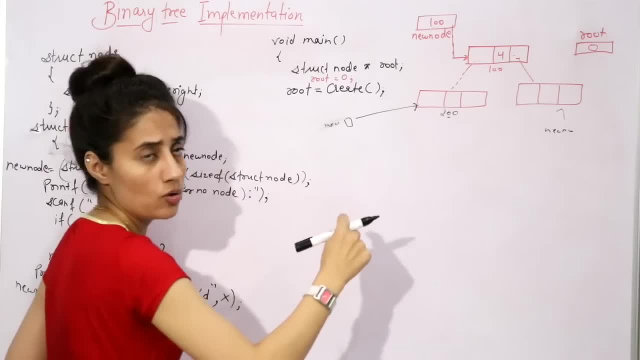 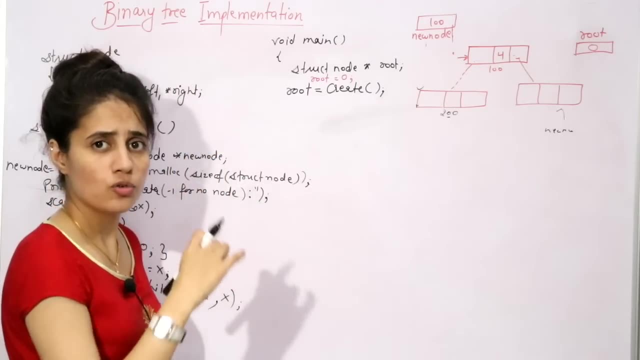 these are what the copies of this local variables. it's not like that, after creating this, this new node would point here and this link would be broken. see this thing: how this recursion and recursion is going to work. this thing also we will discuss in a separate video in detail right now. 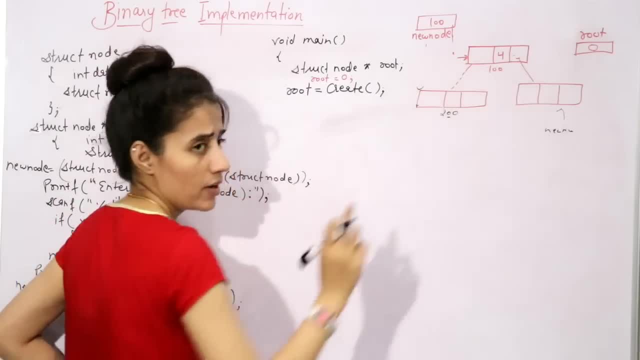 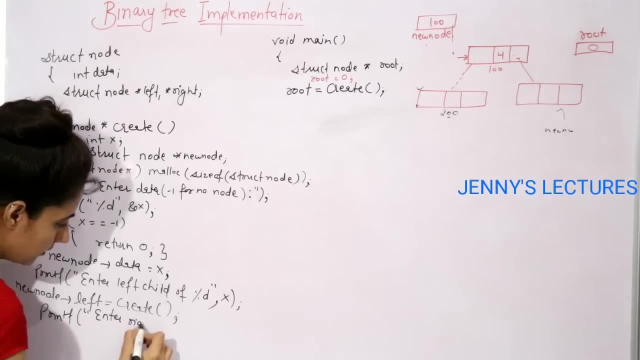 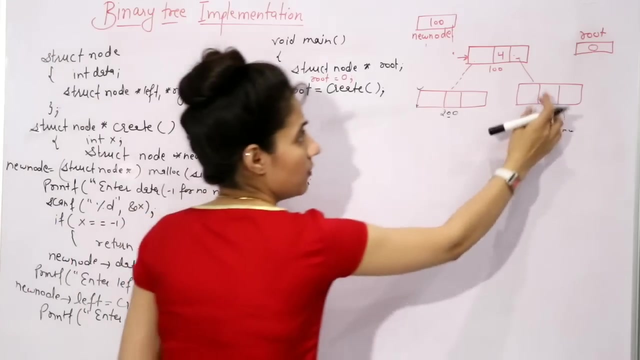 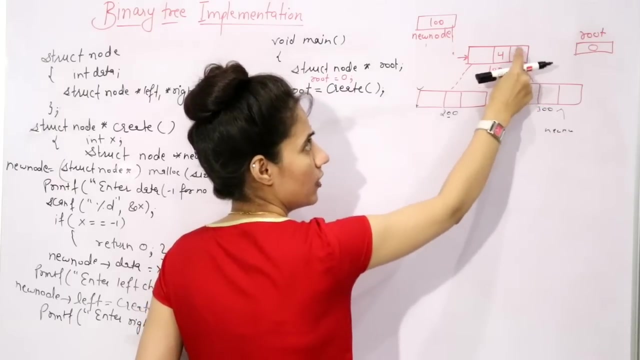 after this left, you need what right child also. so here simply you will ask printf: enter right child of percentage D and here you will print X, right. so here same, you will call create function and what this create function will return here this address of this right child. suppose address is 300, so it is going to return 300, so that I can store here 300, right? 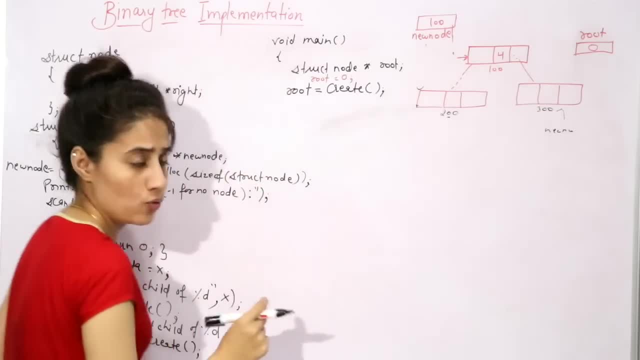 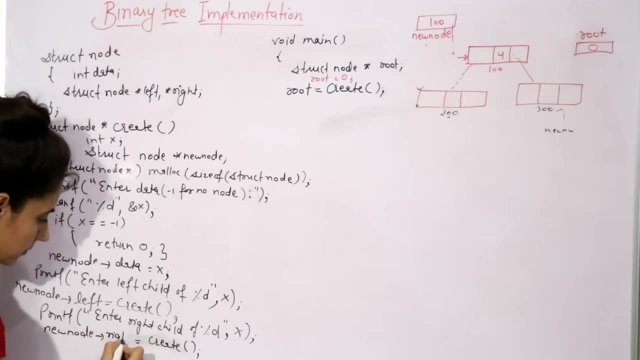 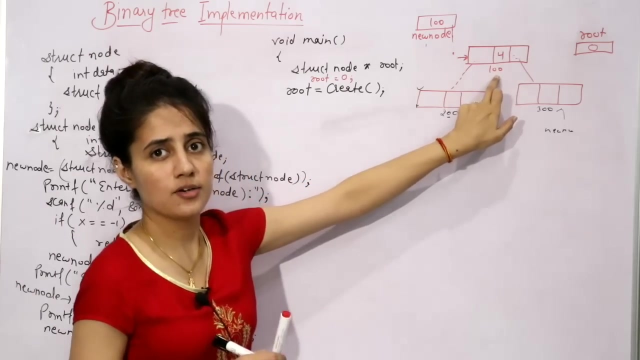 so now how you can access this part- new node, right. so whatever this create will return that thing. we are going to store in new node right in this pointer. and finally, we are going to return this one, the address of the root node, so that I can store this 100 here. 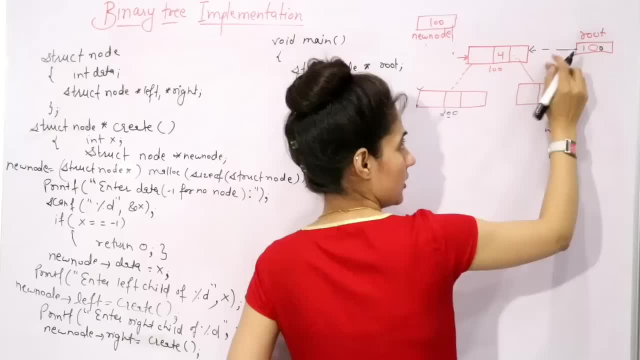 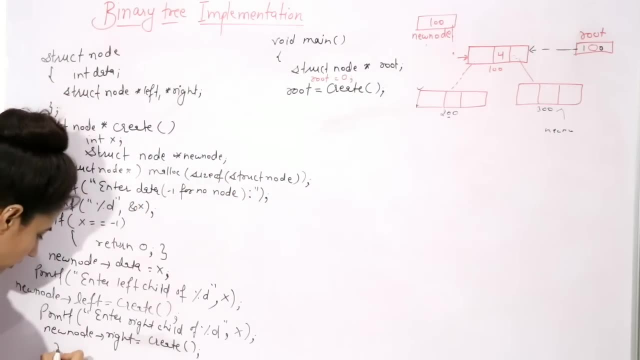 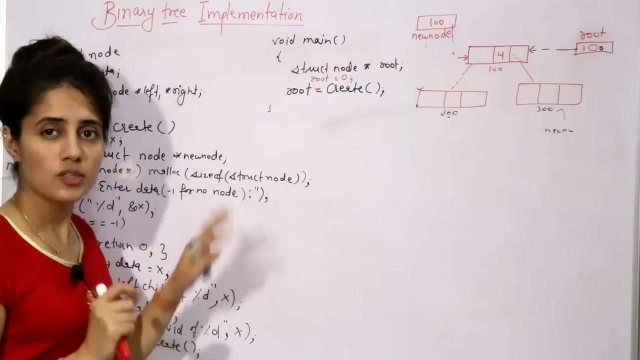 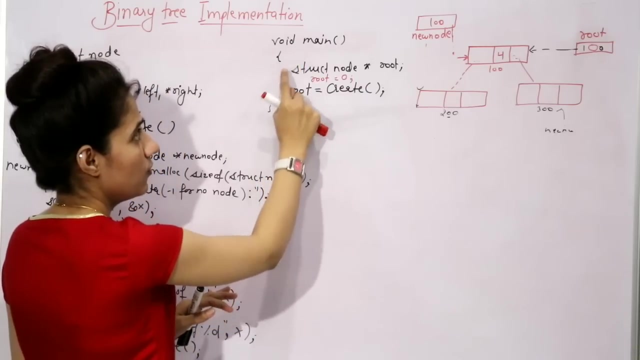 so that this root can point here. and once this pointer is established, we are going to have only this route. pointer value, right. so here. after that you will write return node. fine, now see the working of this code. see, whenever the function is called from the main function, the control will go into the main function. one root pointer would be created. 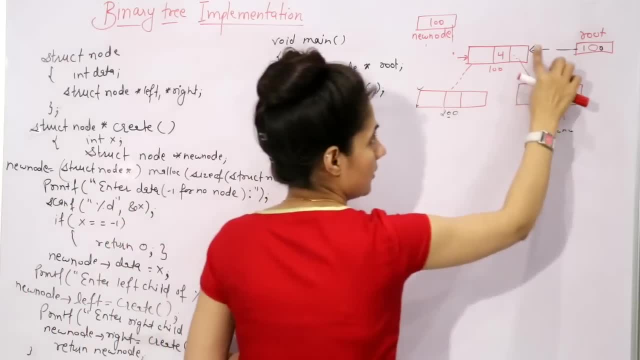 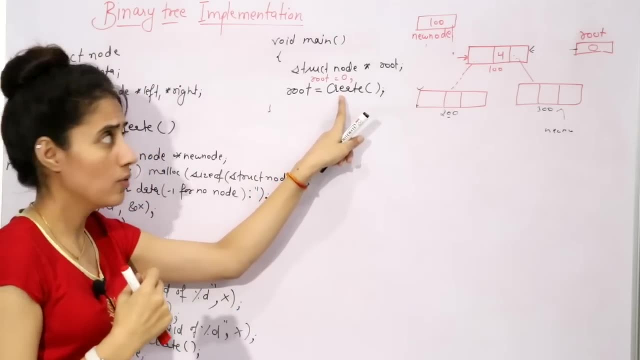 initially we will store here null, right like this. here we are going to store here null. now i am calling this create function. whenever the create function, the any function, is called from the main function, the memory is to be located in the stack right see now. see the working of this recursion. 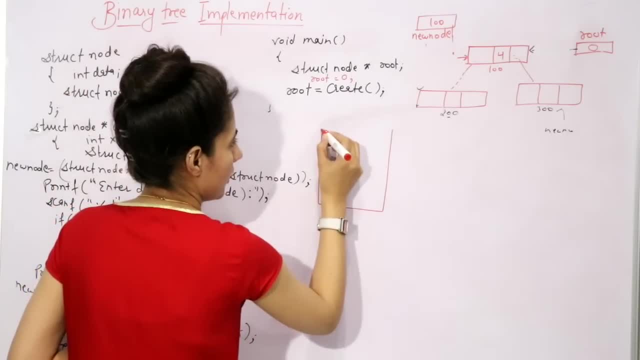 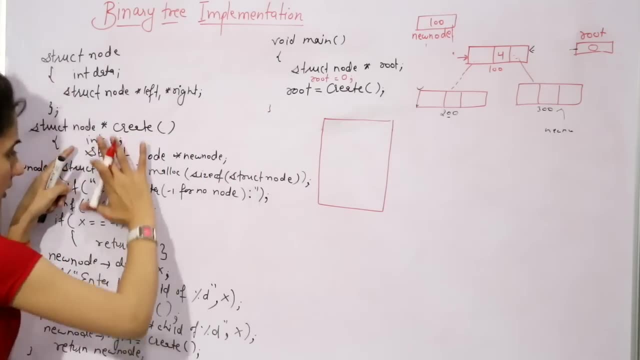 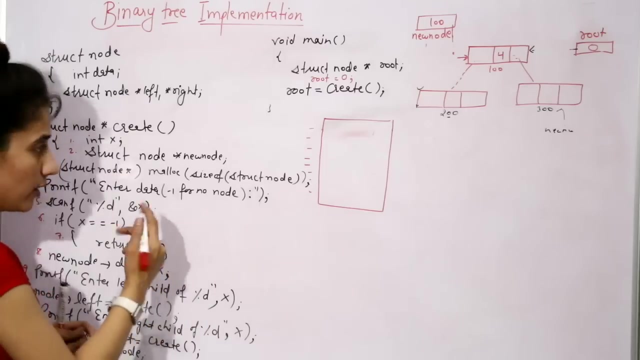 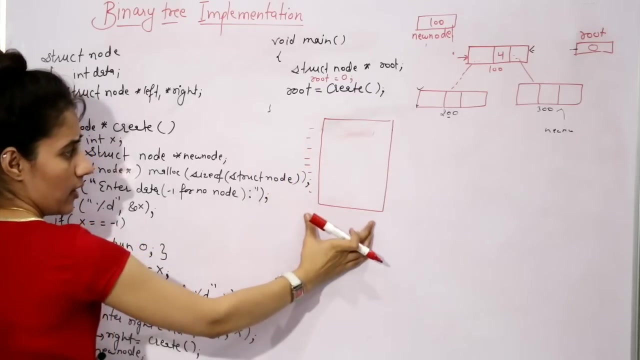 here. suppose i have allocated the memory in this stack right for this create function, so now the create function. whatever the these statements in the create function, these should be copied here, all these statements from here to here. so here i have numbered these statements right, roughly, i have numbered all these statements would be here in this stack the memory has been allocated for. 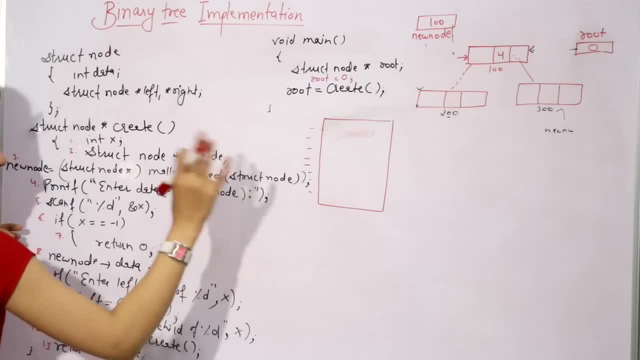 this create function in this stack right, so mainly i am writing the memory in this stack right, so i am writing the main main statements here. this two statement means this new node would be created right, as we have discussed here. the third statement in the third, this dynamically. 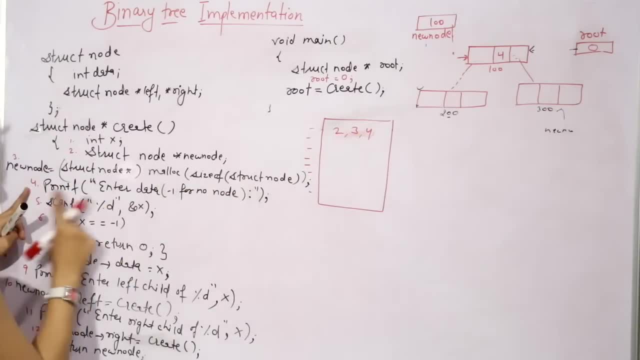 memory has been allocated. we have entered the data, that is. this is the fourth statement. this is the fifth statement. we have entered the data x. now i have checked six. if x is equal to null- sorry- minus one, then return zero. but here i'm entering four, so this condition would not be executed. 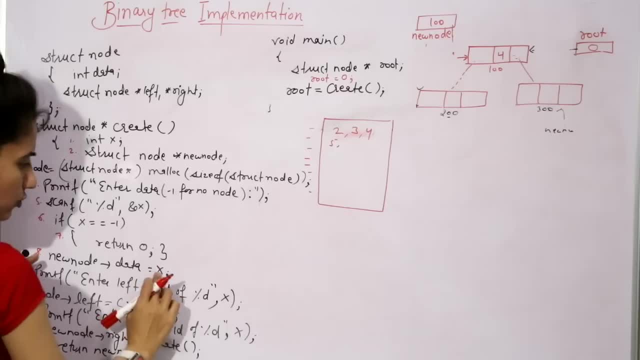 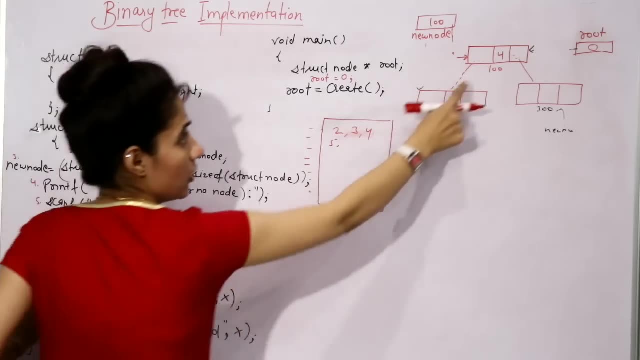 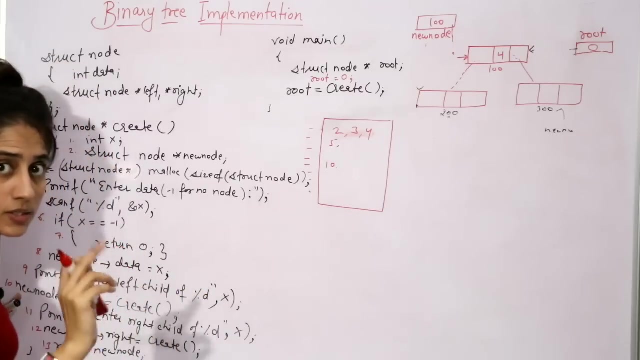 this statement would not be executed. now new node data and x is equal to x, so i have put here four. now see: enter the left child of x means enter the left child of four. that would be printed right now. this statement, the tenth statement: see now x. this is the sixth statement. this one, six, seven. 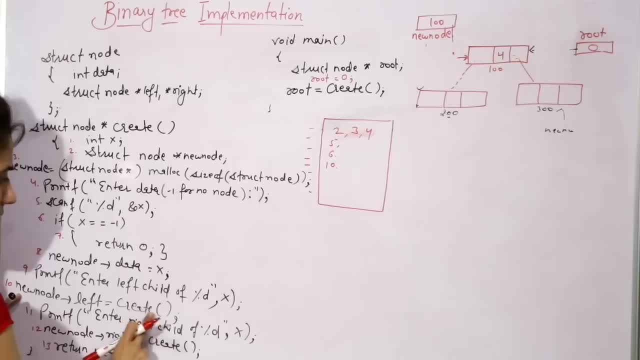 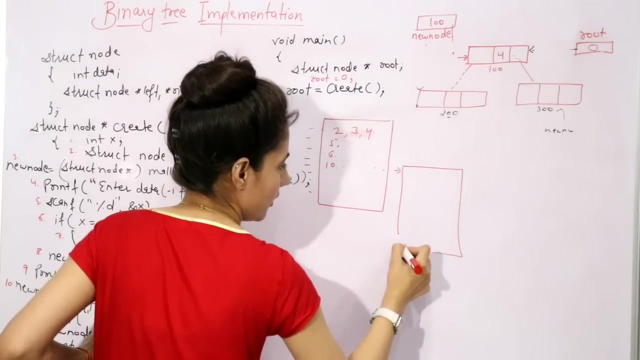 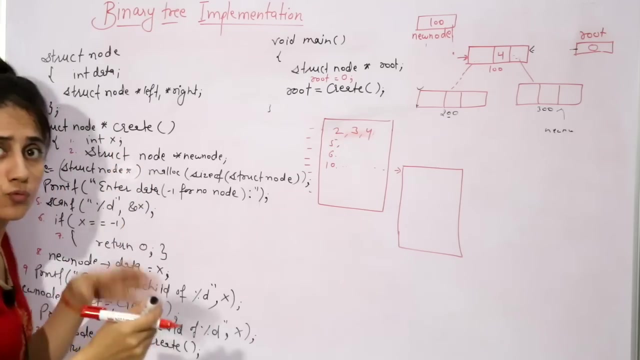 and you can say eight. this is what tenth statement now again create. so from the tenth statement again we are going to call create function means again this: you can say: stack would be there again. all see, different copies of these local variables would be created for each function. 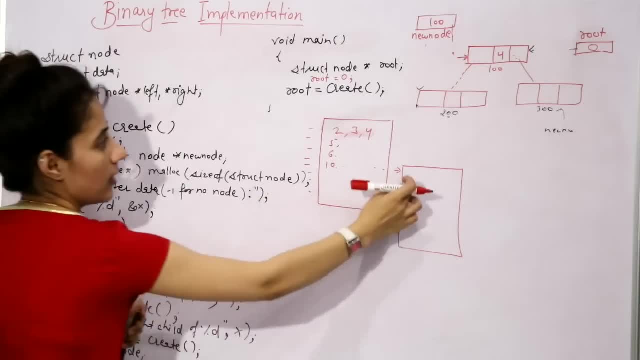 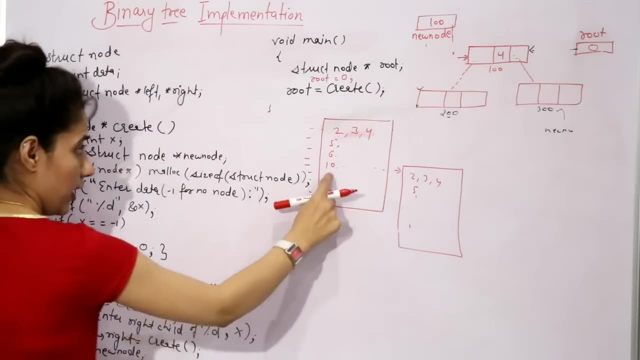 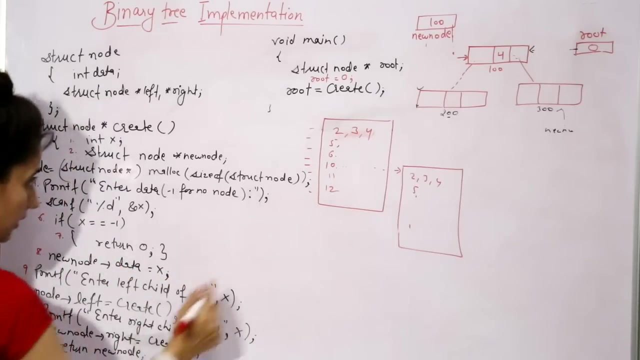 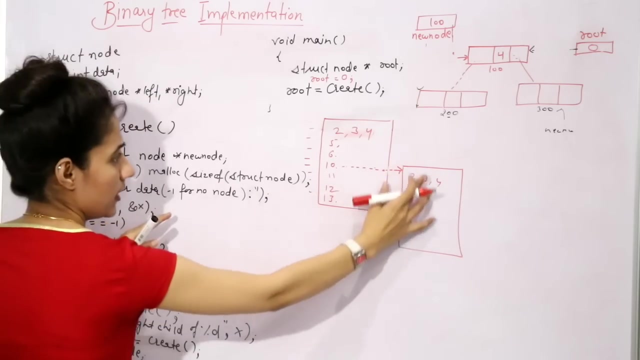 call. so here also all the statements would be there. you can say one, two, three, four, five and up to 13 statements right now, here also we have see, after this tenth statement we have 11, then we have 12 statement, right, and then we have 13 statement. so now see, in this call again, all the statement would be executed. 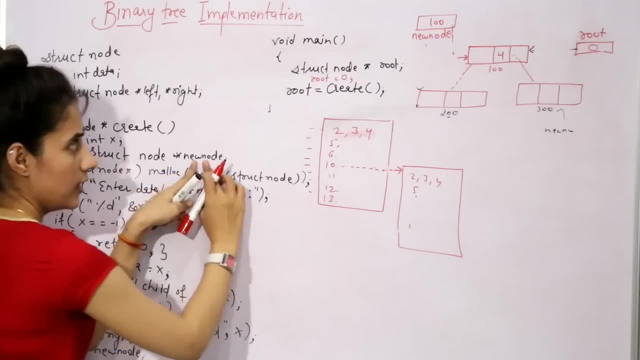 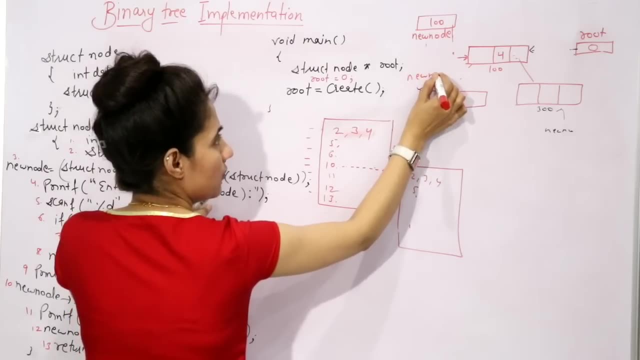 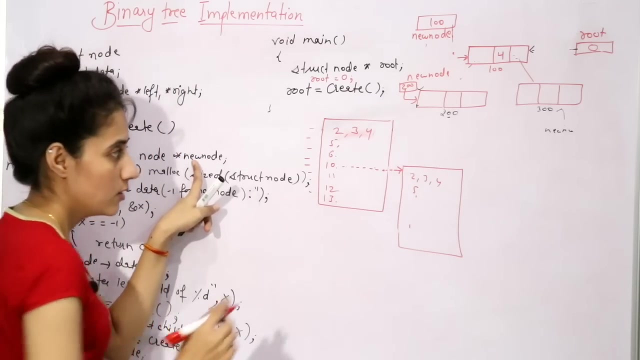 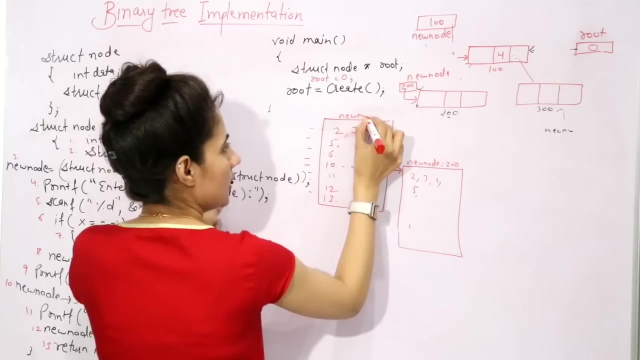 here right again, this new node is to be created. so now, here suppose i have created this one, this new node. so now, here also i have a different copy of this new node. pointer: suppose: this is 200, so here i have 200 right. so here you can say: here also we have new node, is 200 here? in this case, new node is: 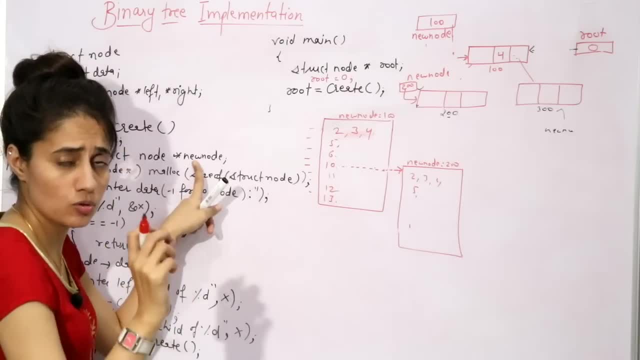 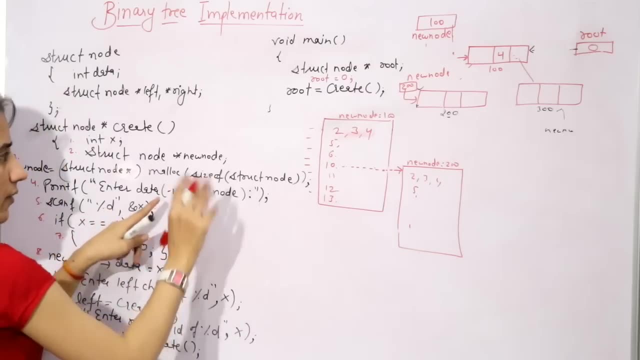 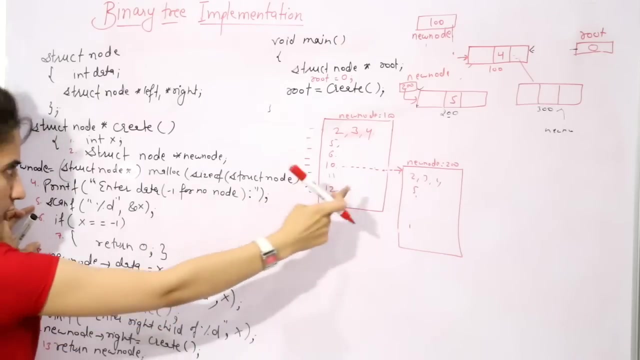 having 100. these are two. you can say copies of the same variable right for different function calls: fine, now memory is to be created. minus one. we haven't entered minus one. suppose I want to insert some data. I want to insert here five right, so these statement would not be executed here again. 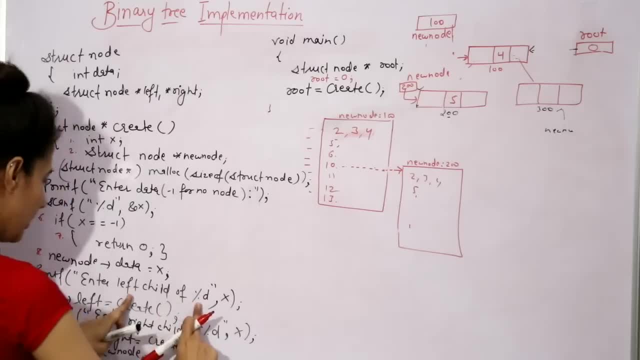 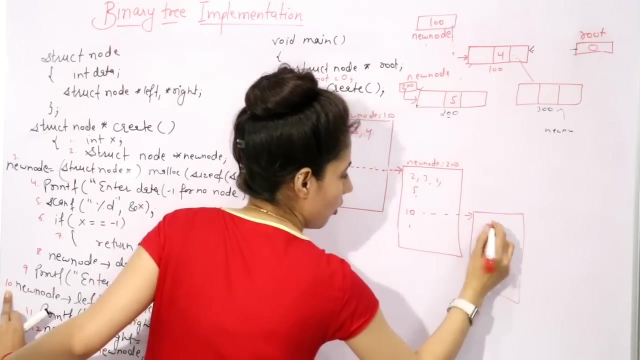 would be entered here. now again it will ask for the left child means the, this one, the ninth statement and the tenth statement. so here again in the tenth statement I am calling create function. so here again I am calling save all. the statement would be executed here that this create function in this. 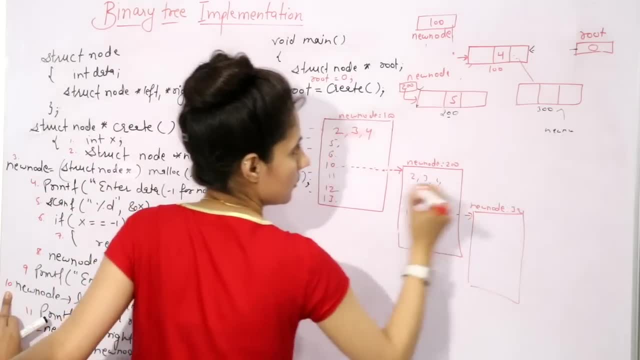 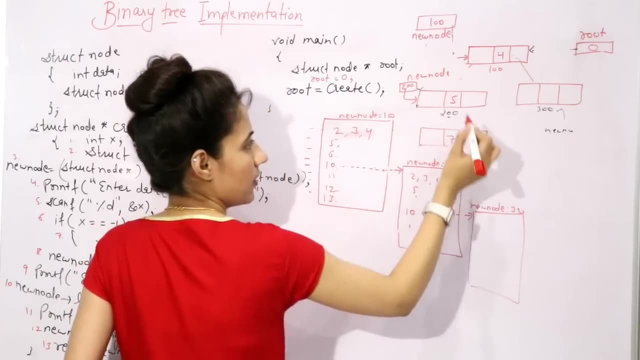 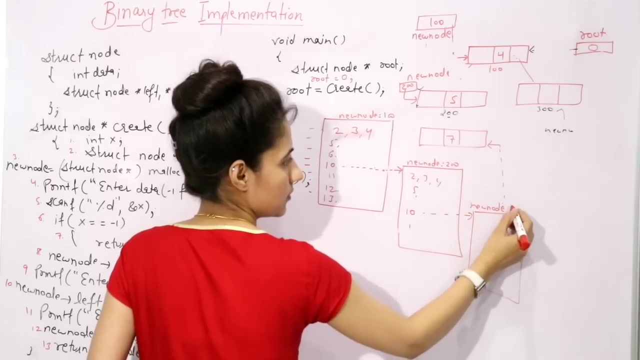 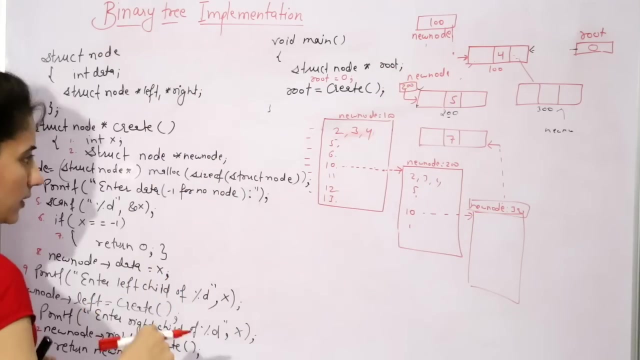 case. suppose here I have new node is equal to 300. here I have created a new node, right, and here I want to store seven. fine, now in this case new node is having 300, so this new node is pointing to here, right, this new node. three copies of this new node I have now, as you can see, see. 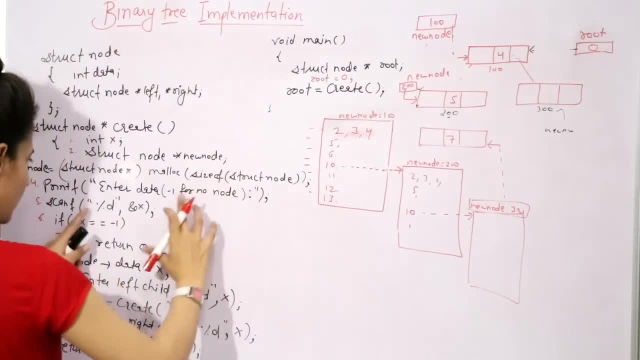 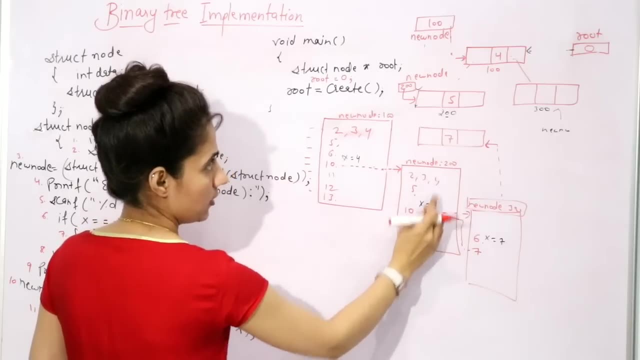 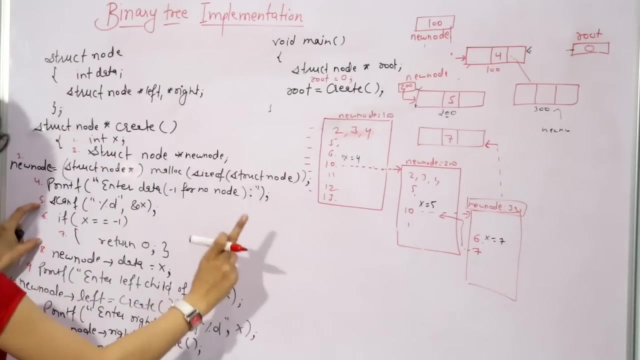 here, suppose 300, same these statements would be created now. see here: the x value is seven, because I have entered seven here in this case. at this case I have entered five and here I have entered four. right now I have entered seven. it means these statement would not be executed. now again, enter the left. 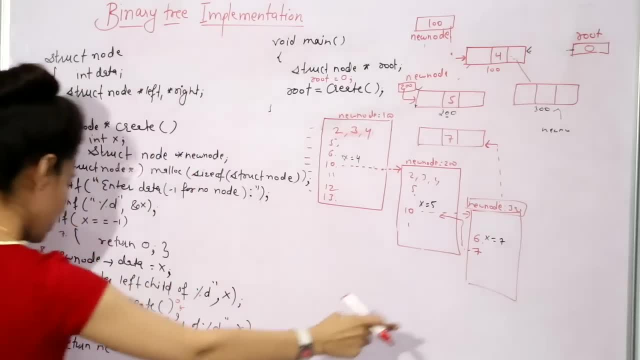 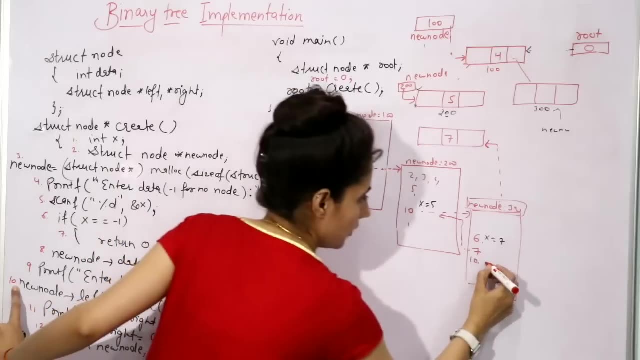 child of x. the ninth statement in this stack would be executed now. at the tenth statement again, create function would be called. right here you can see: create function would be called now, again the calling of the create function: now same. the all different copy of these local variables. 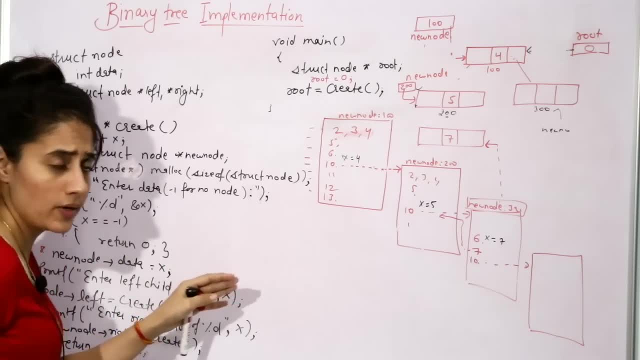 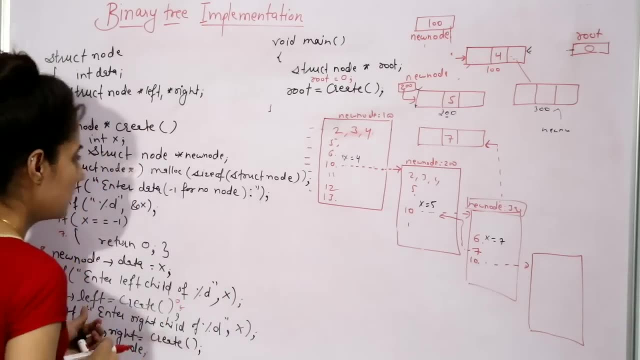 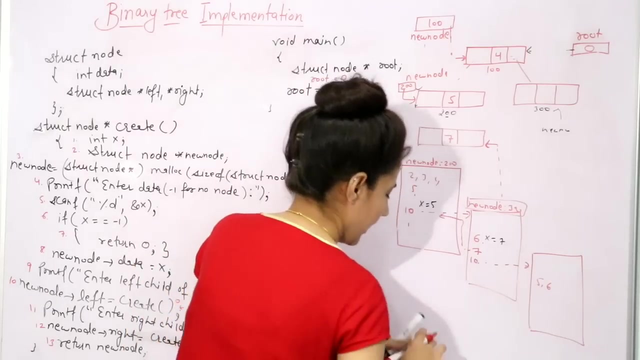 would be here, created in this stack for each function, call right. so here also all the these statements- 1, 2, 13 statement- would be there. now we will see the execution. now suppose here this new node would be created. but here I have entered. at the fifth and sixth statement I have entered what 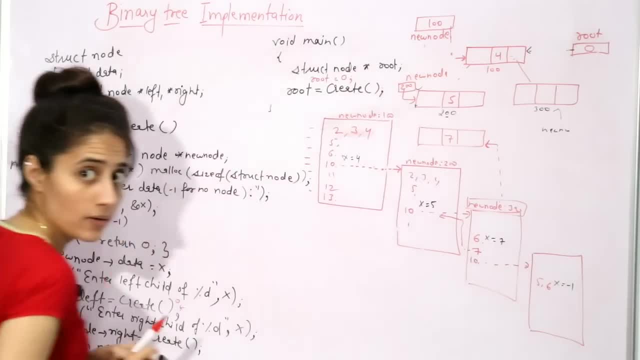 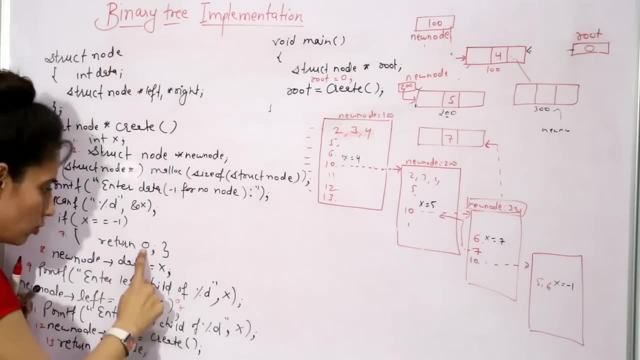 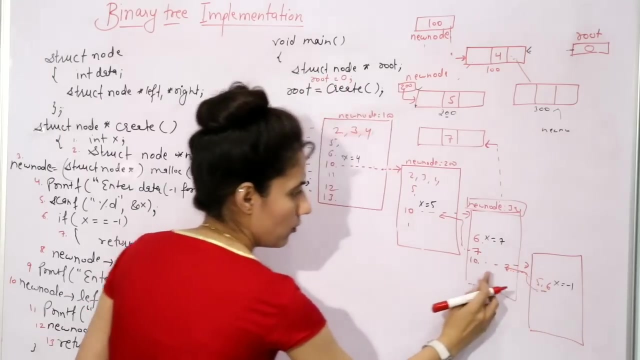 x value is minus 1 right now. if x is minus 1, then the control will go within this. if statement means return 0, the control will not execute these statements, right, because now this statement is true, it means it is going to return. return means here, where you have called, here I have called in the. 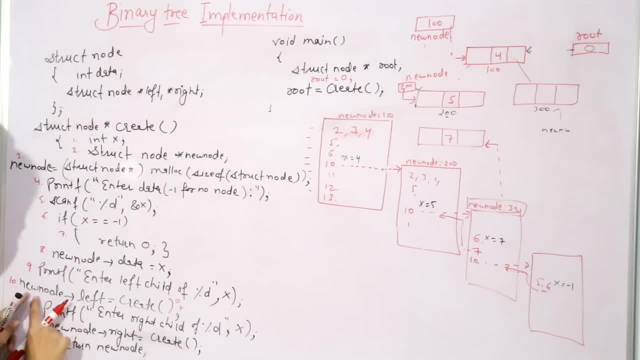 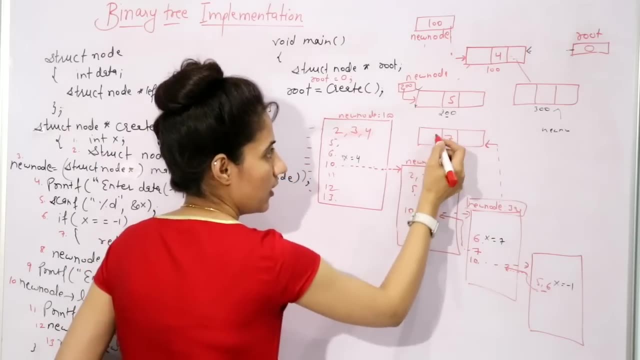 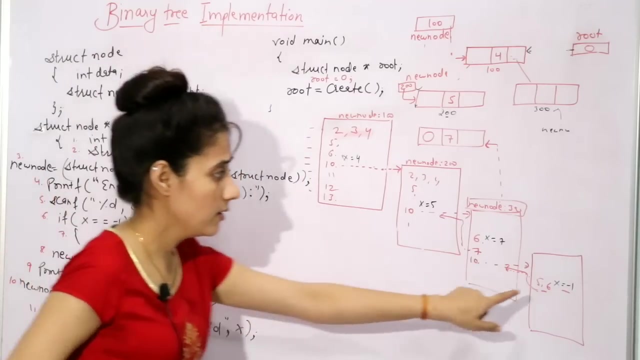 previous stack right, so now it will turn 0. that would be stored in new node left, so here it will return 0. here. in this case, new node is worth 300 means here, so new node left, here I will store 0. now see here: this is what the base condition when x is equal to minus 1, from here you need to return. 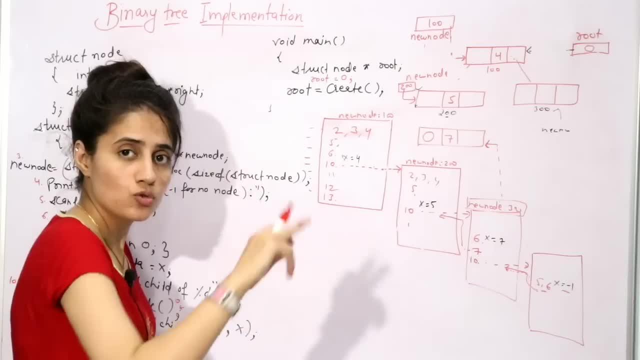 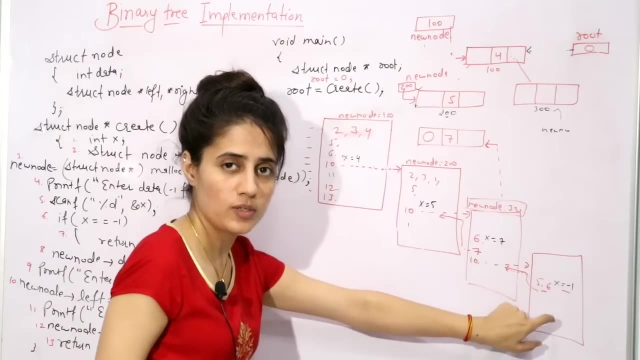 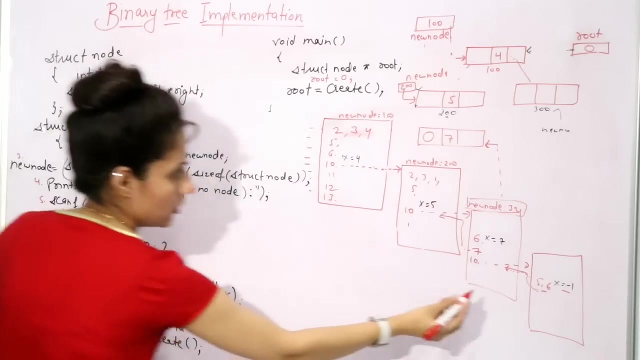 once the base condition is raised from there, the function is going to return the value where it has been called right, and then the memory has been destroyed from this stack and this process continues right. so now, here I have written here 0. now the control is here. I have returned the value here. now, after 10, here I have. 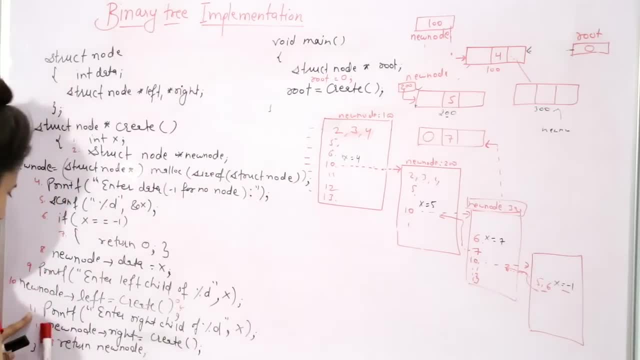 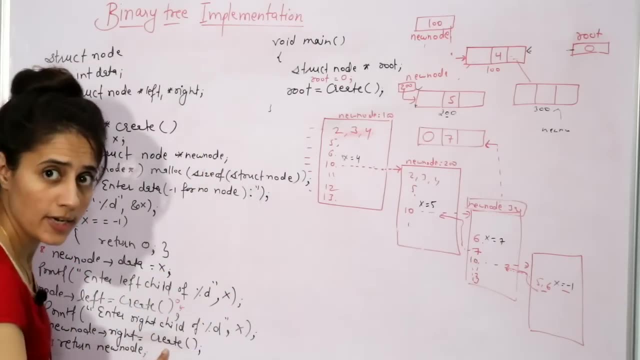 11, 12 and 13. statement 11, 12 and 13.. now enter the right child of x. here x is 7, so enter the right child of this, 7.. again, you are going to call create function, right? suppose I am calling again here. see here at the. 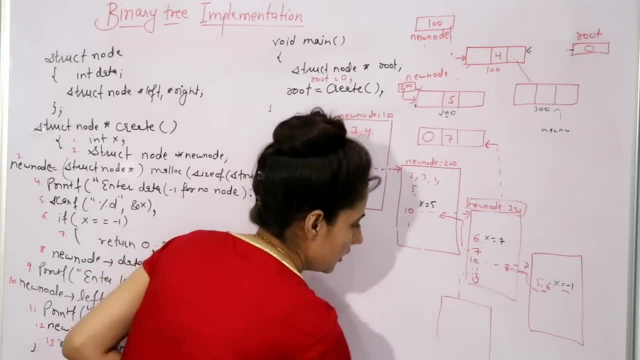 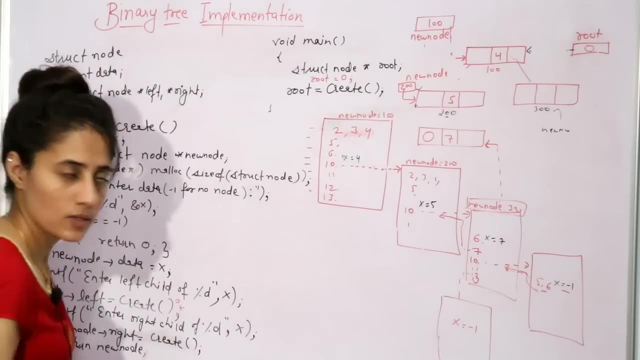 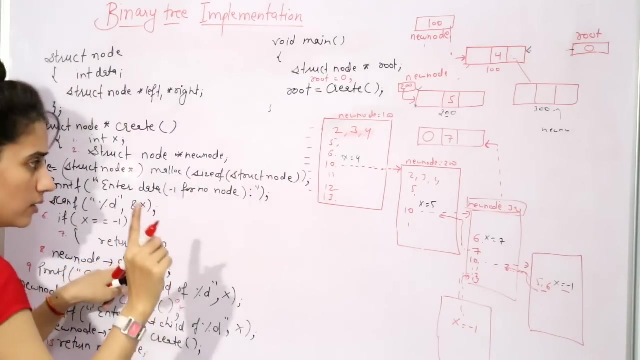 12th statement. at the 12th statement again, this create function would be called right. one stack would be created. now suppose here I have entered x is equal to minus one, same in this case. so it is going to return back to here. right, it is going to return what? null and. 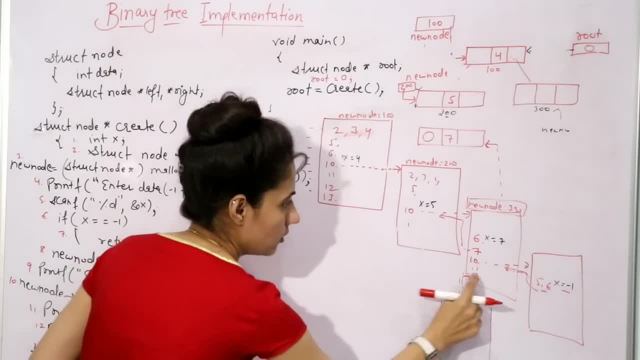 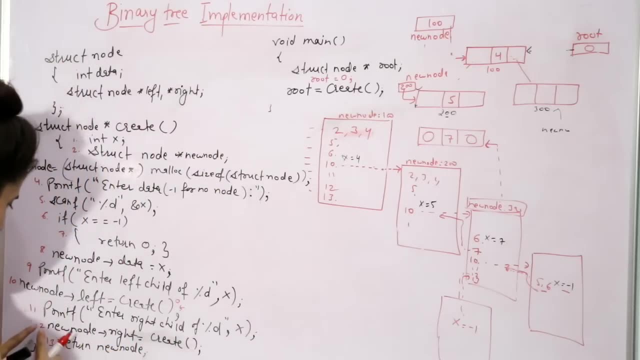 whatever it will return. we are going to store here new node, right, so it is going to return here. here is 300, 300, right, here you will store null. fine, now, after these statement, after the 12th statement, the 13th statement, control will go to here. now, in 13th statement, you are returning what return. 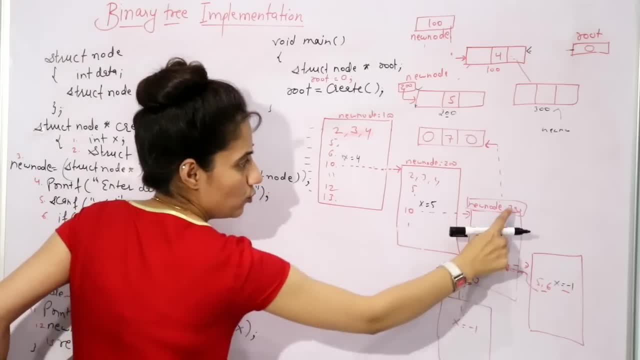 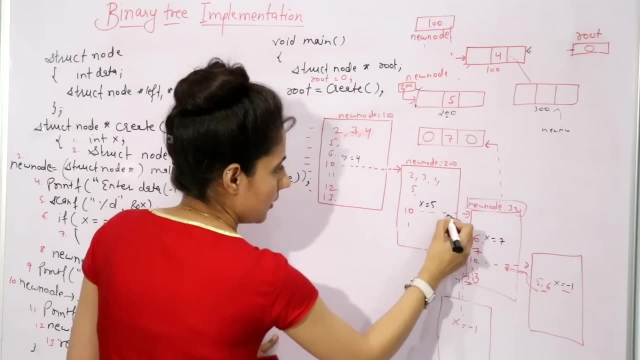 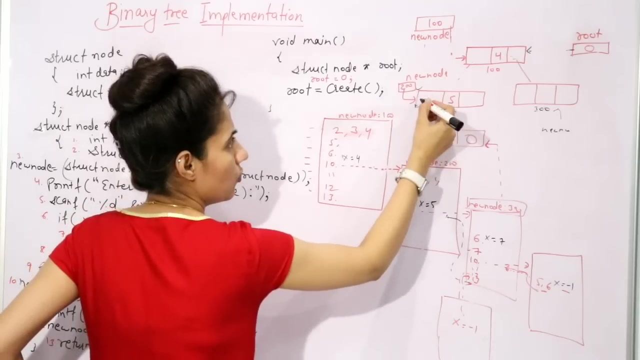 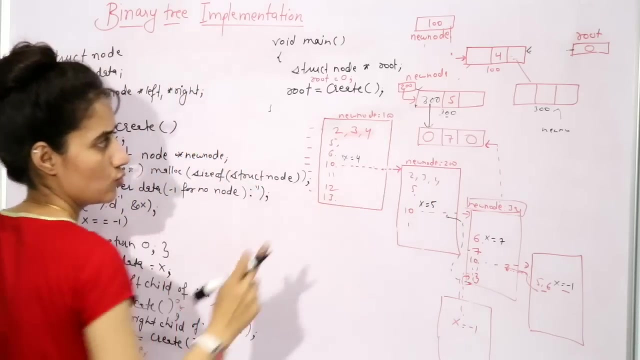 new node. now it will return what new node, that is, 300 would be returned, where the 300 would be returned here, back here, because here i am calling this function: right so now, 300 would be returned, so 300 would be stored here. right so now, this is what the left child of this one, fine, now see. 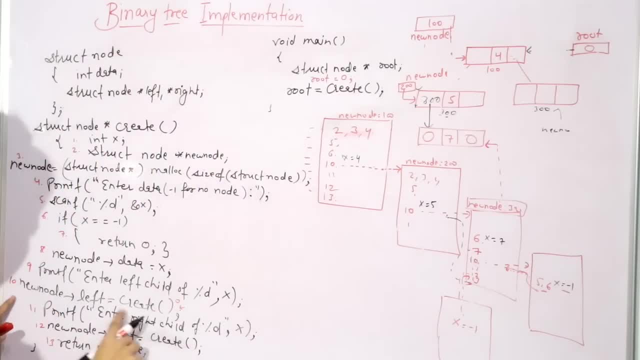 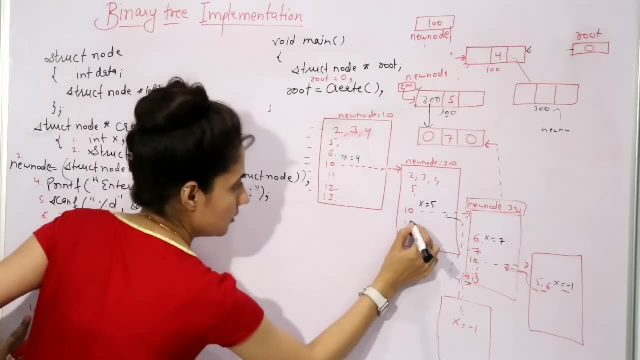 after returning of 300 here. after 10th statement here. some statements are there which are still not executed. right means this one: 11th, 12th and 13th. 11th, 12th and 13th: we'll ask for the right. 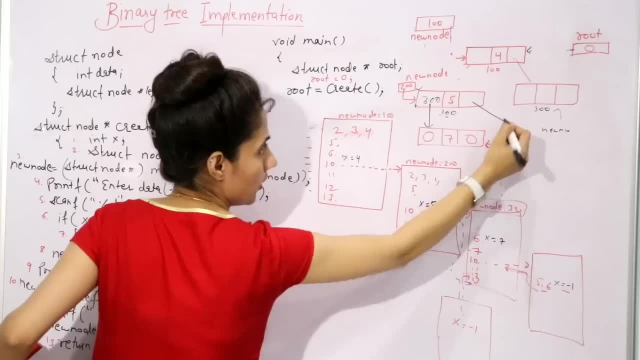 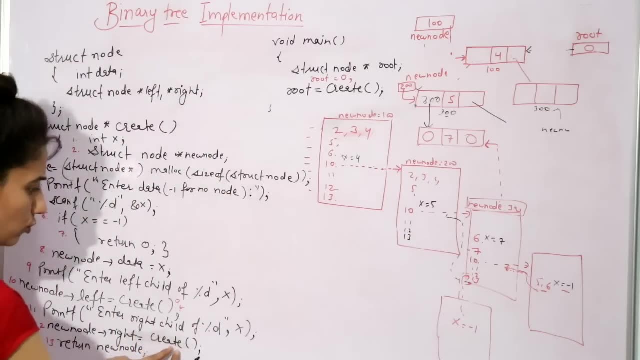 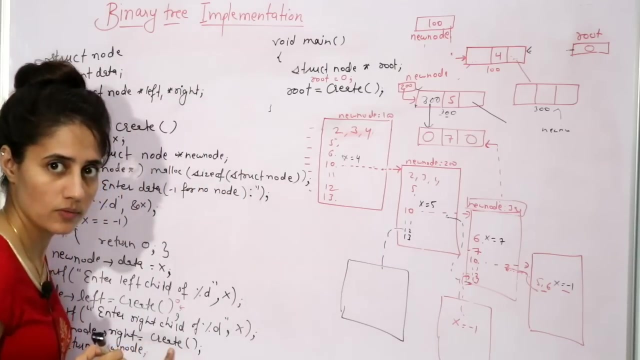 child of x. here x is 5. right child of 5 means this one right suppose. right child of here x means it is again going to call create function. so here this 12th statement is again going, again going to call create function, right suppose, here i am. 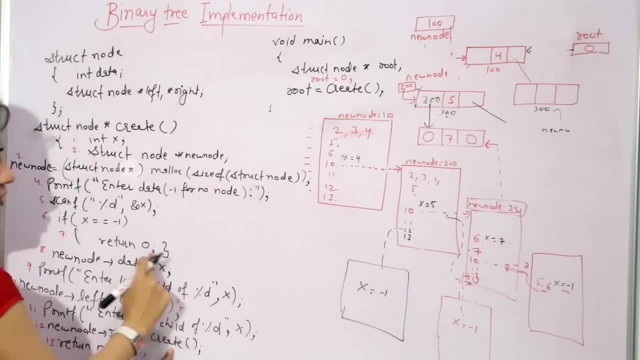 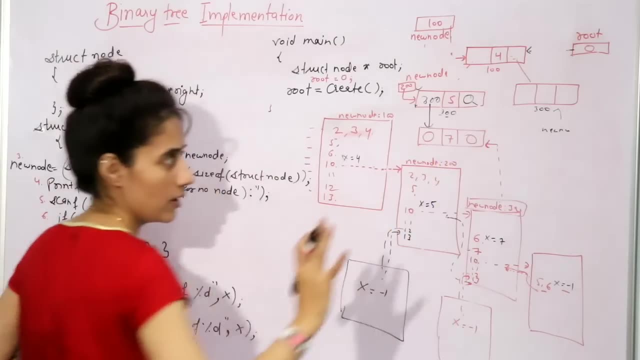 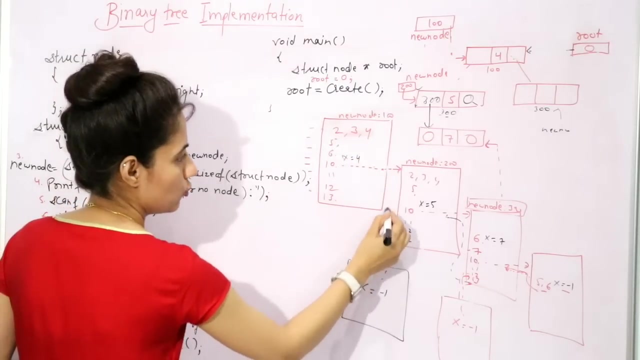 i have entered. x is equal to minus 1 means here the return 0. it is going to return 0 here. fine, so now, here you will store 0. there is no right child right now. after this 13th statement, it means it is going to return here. because here i am calling this, this function, here this is the. 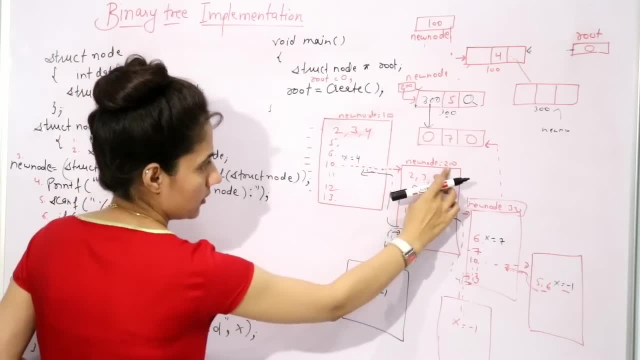 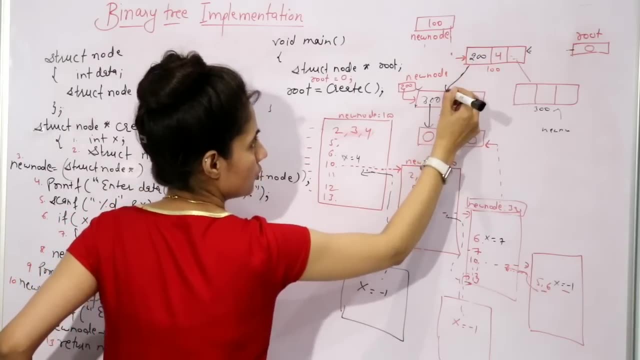 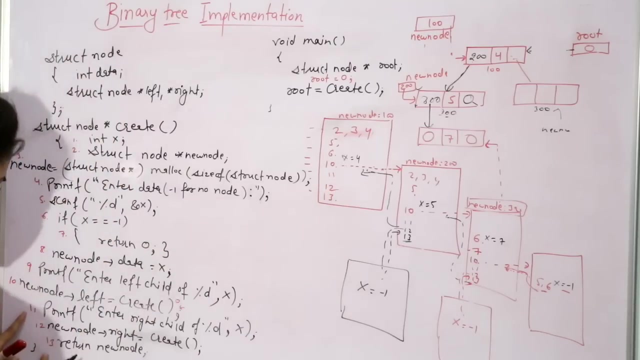 function call, that is, it is going to return what? 200 return new node. here the new node value is 200, so it is going to return 200, so here you will store 200. so this is what a link to here. that's exactly we want right now. here also 11, 12 and 13 statements. 11 is right, child of x, so here again, 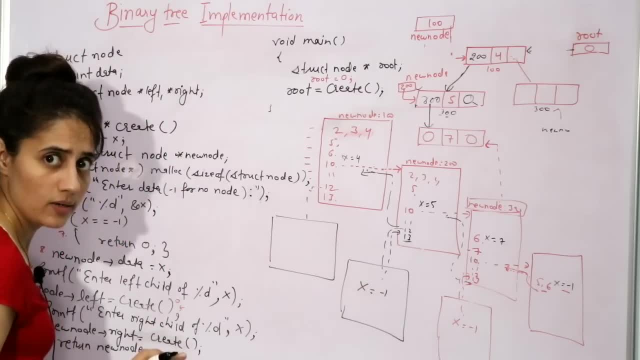 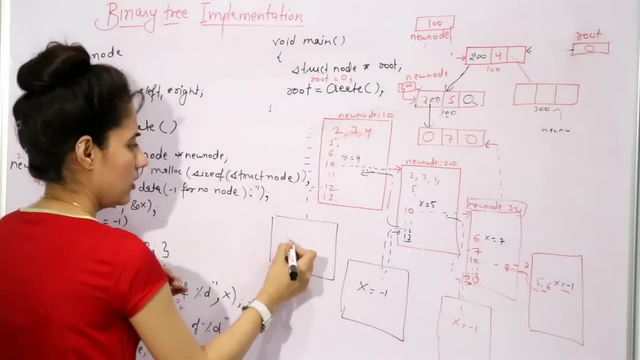 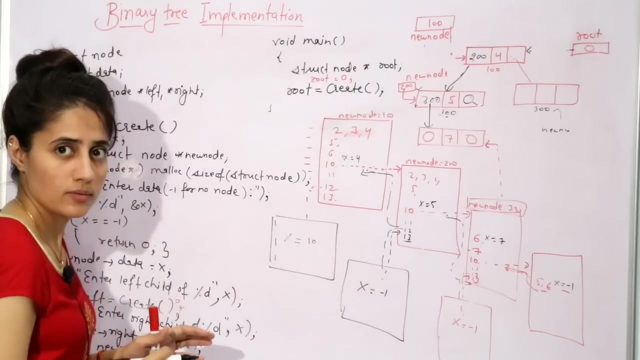 going to call that create function, right? and suppose here also you want to create here this new node, you want to insert some value, so here you can insert x value is you can say 10, fine, so here also same execution would be there that i have discussed here. right, this is just. 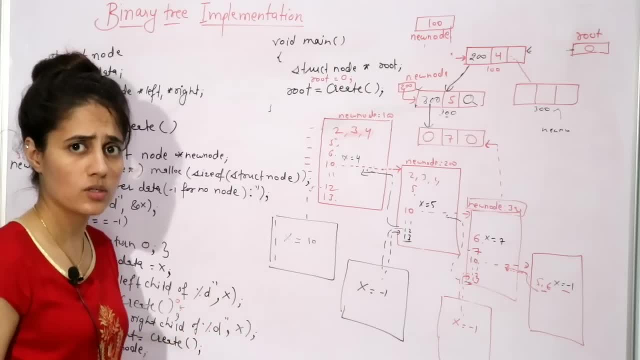 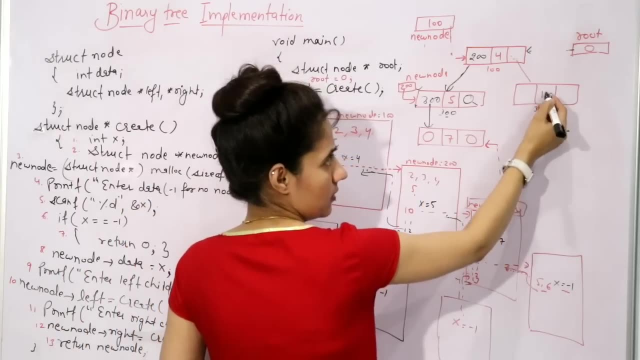 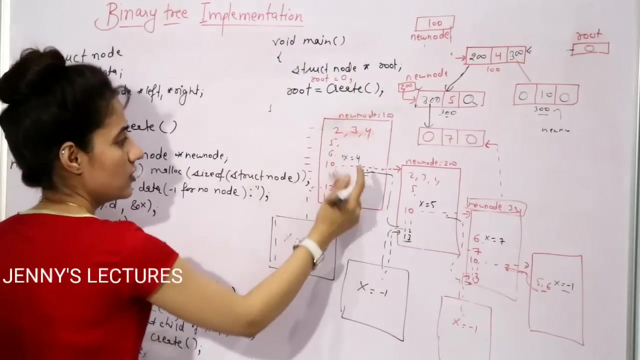 a brief of how the recursion is going to work. this thing we are going to discuss in detail also. right, the working of recursion. now see here, suppose i am entering 10, null, null. so this 300 would be returned here, right, and at last, at last, when. 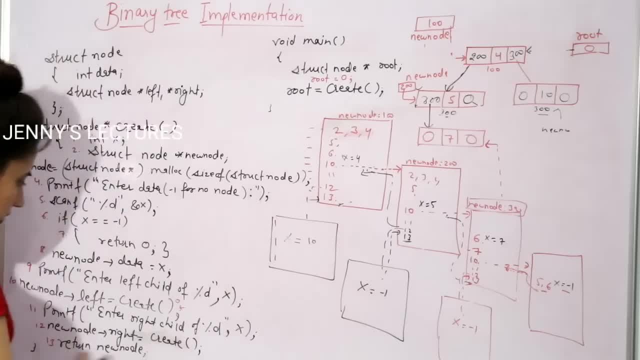 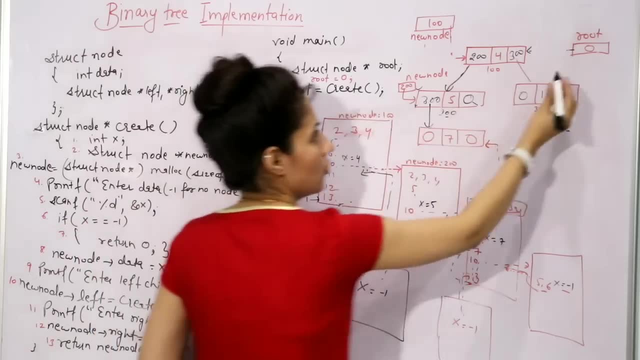 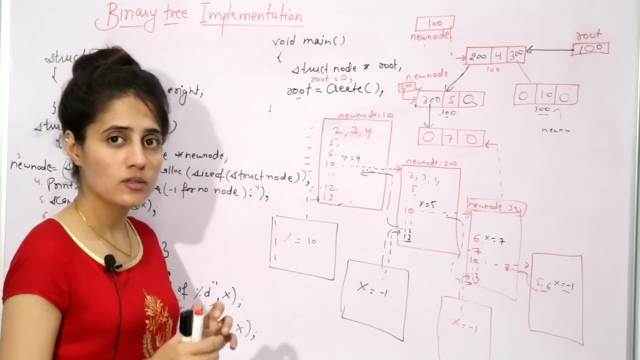 after these returns 13. here also, this return new node means 100. the 100 would be returned finally. so this 100 would be stored in new node. so here you will store 100. so this is going to point here. so this is the implementation of binary tree using recursion. now here, if you want to know that. 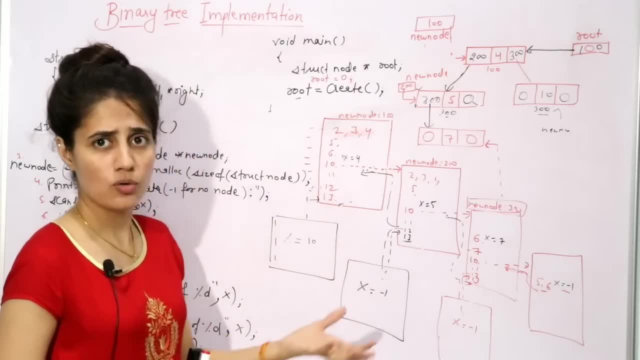 you have inserted 100, so here you will store 100, so this is going to point here. so this is the implementation of binary tree using recursion right and here you can see that you have inserted 100 employees, a Style procedures which is going to control67 solution right and if full.